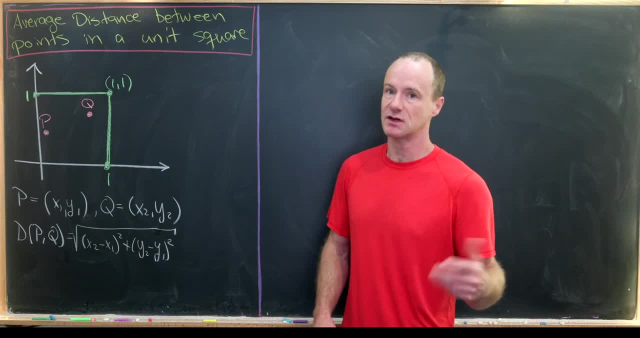 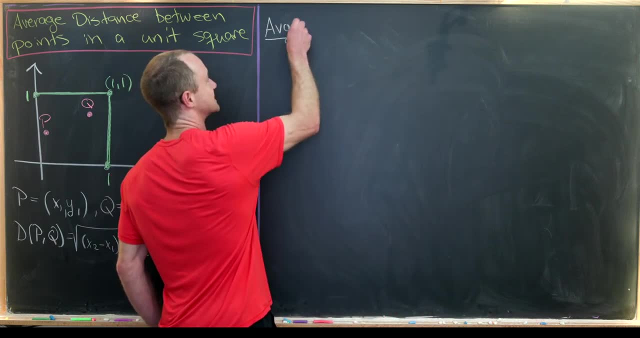 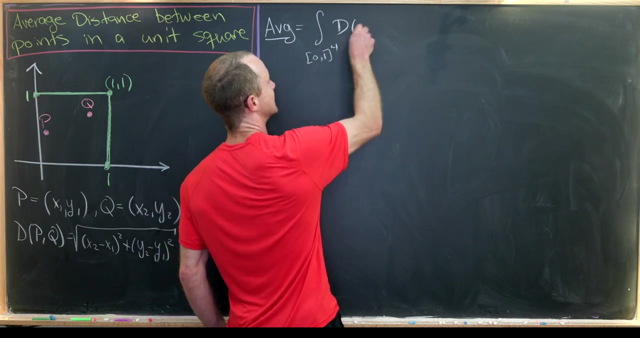 Luckily that's really just equal to one, because it's one times one times one times one. Okay, so anyway, let's maybe write that down. So we've got this. average is equal to one times one times one to the integral over. I'll write it as zero. one to the fourth power of the distance between p and q. 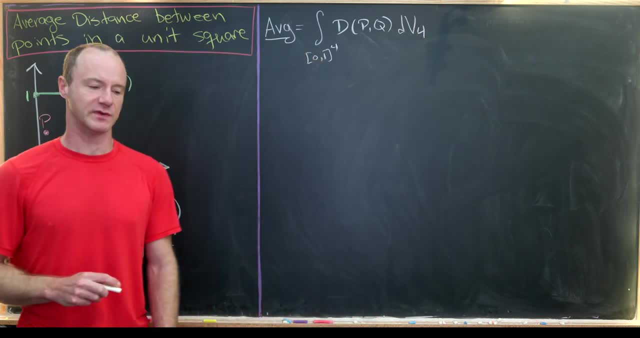 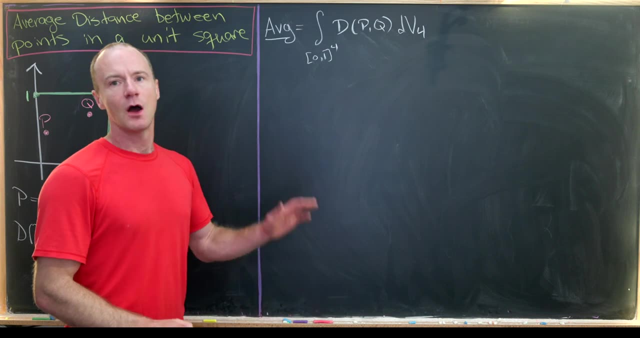 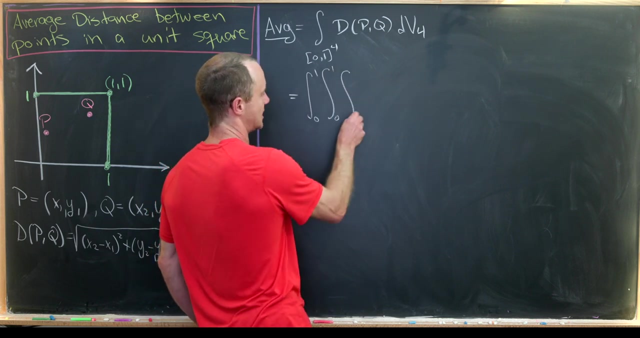 and then I'll just say d v, four, So that's like our four-dimensional volume component, where of course this d p q is given by this down here. Okay, so now let's write that out a little bit more extensively, So that'll be the integral: from zero to one, zero to one, zero to one and you. 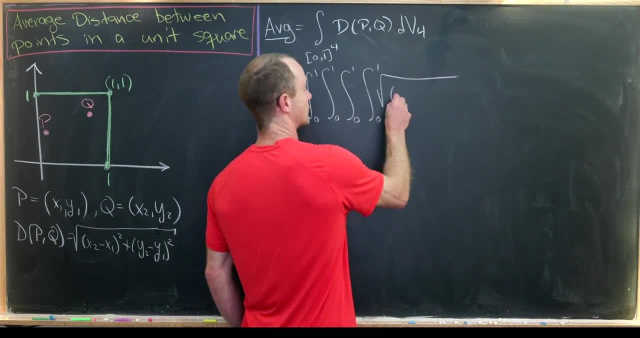 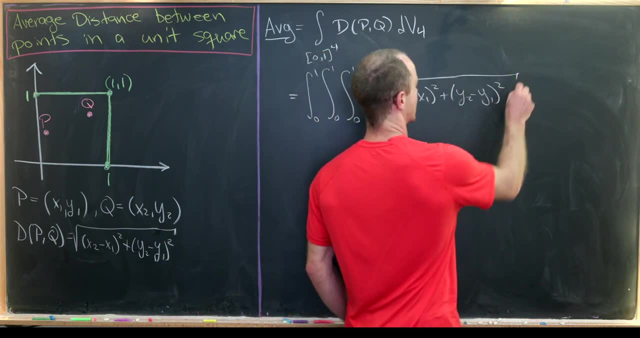 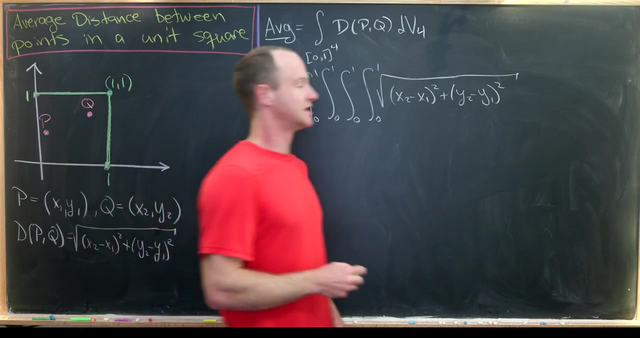 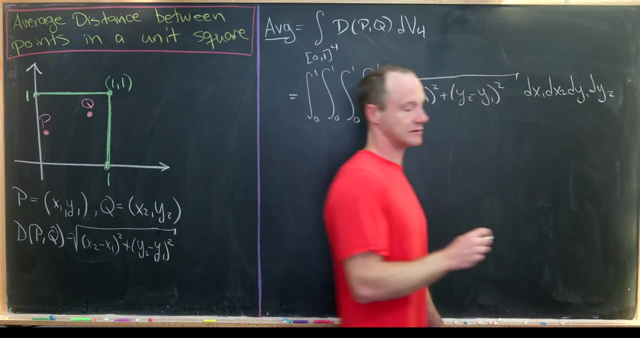 guessed it, zero to one. So that's equal to the square root of x2 minus x1 squared, plus y2 minus y1 squared. and then this differential volume component- since we're like working with rectangular coordinates, can be done with d x1, d x2, d y1, d y2.. So I think you can already see why this very easy to state problem. 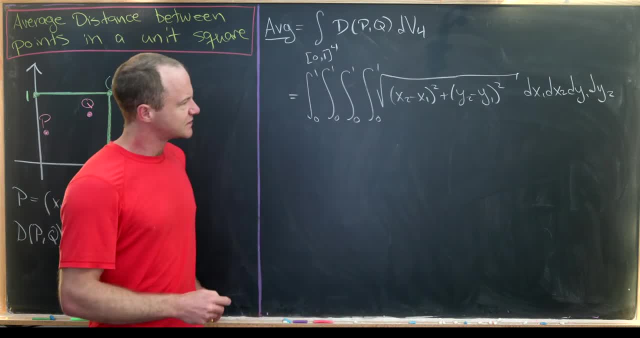 is actually quite nice, So I'm going to go ahead and write this down, So I'm going to go ahead and run this. So I mean, the first thing that we're doing here is actually chain some Help Wort next, but one of the last things that we're going to do is a rule down here. So this is thehalt of Y. 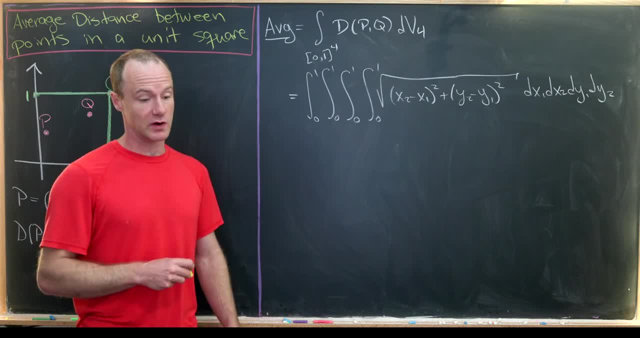 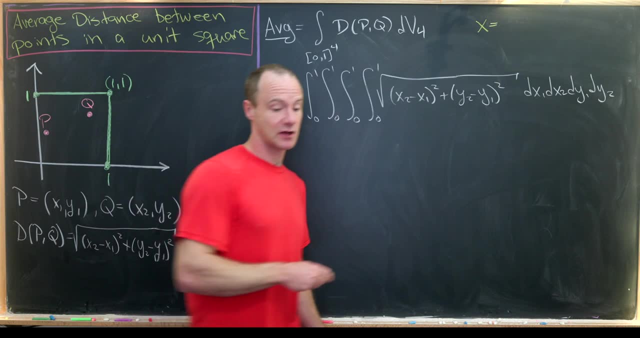 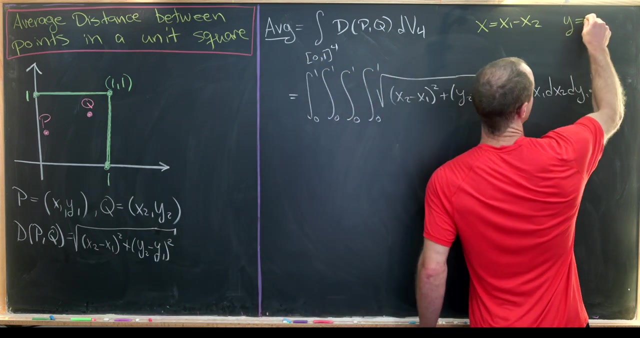 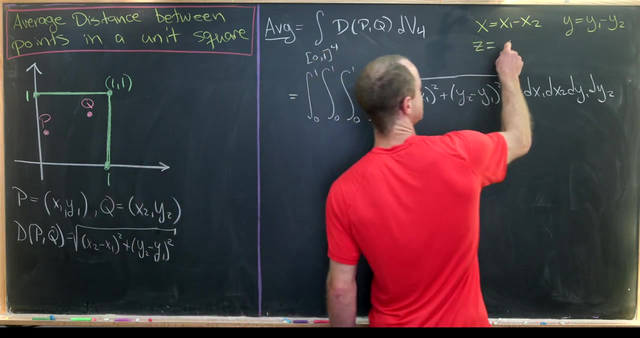 created by our helpful roommate. If you不好意思, but if you know where that was, it's X. so Y is X, but Y is Y. that's a different thing. If you need to guess, let's help, Cause we already know X because we got some length died here. X will be 0 because right now we do. 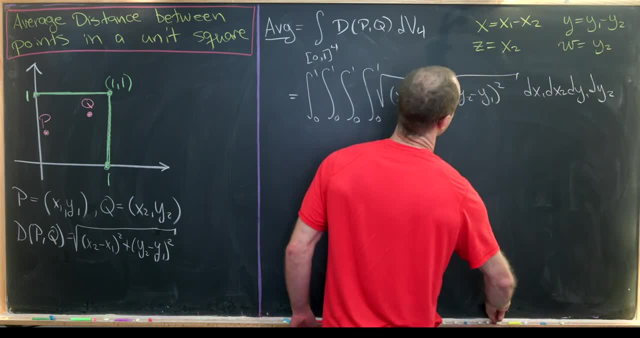 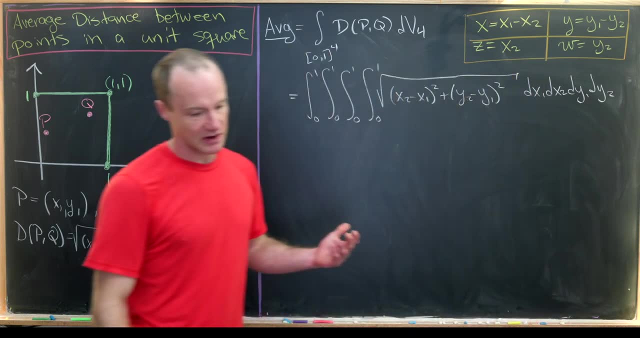 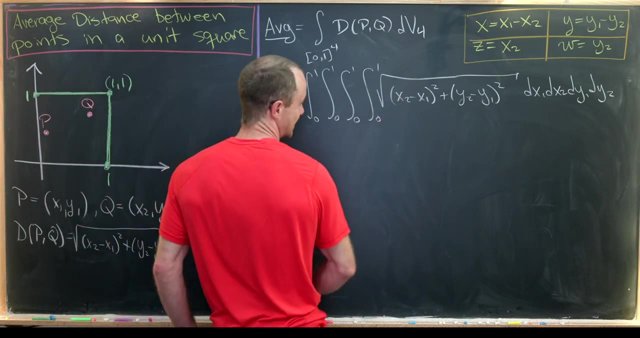 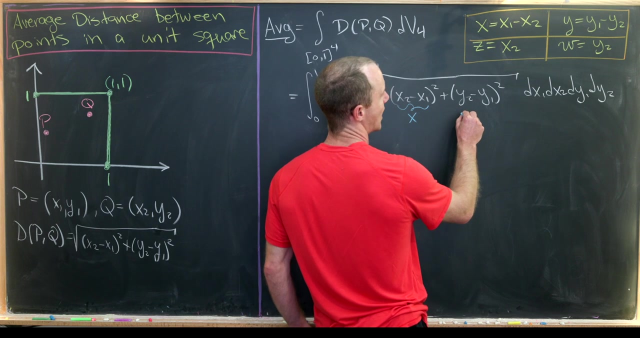 to y2. okay, so that is looking nice. so now, using some rules about change of variables, we know that this should be equal to well, this guy with the variable changed. so that means this is this: X 2 minus X. 1 will become X. this Y, 2 minus Y. 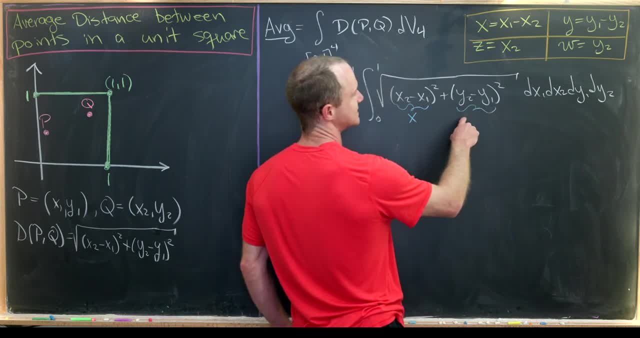 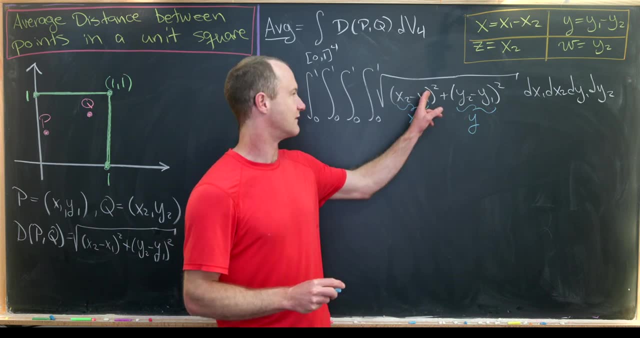 1. well, that's gonna become. let's see why. notice, you might say those should be negative X and negative Y, but it doesn't really matter here, because we have these squares in here. so that's what's gonna happen there. and then we'll also have to. 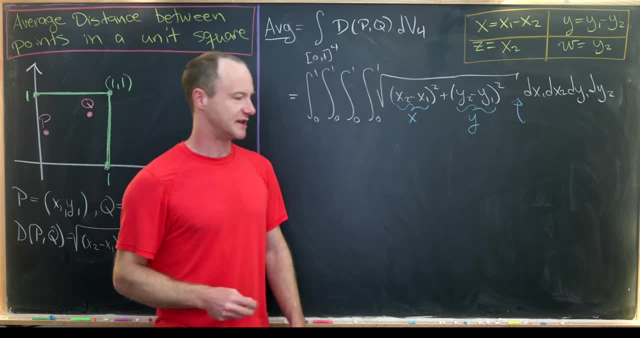 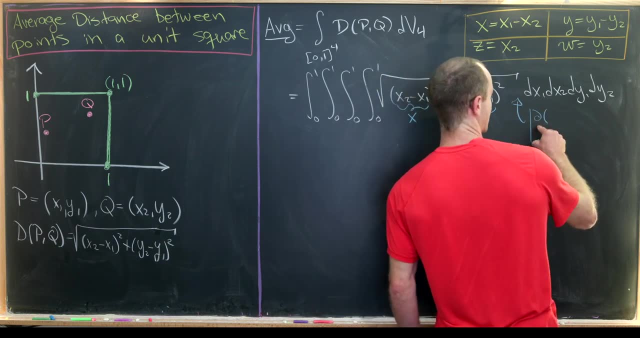 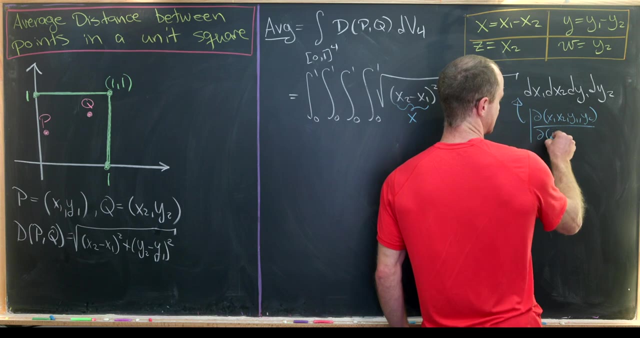 it's set up something or include something, known as the Jacobian, which is the determinant of the matrix given by the partial with respect, or the partial of X, 1, X, 2, y1, y2 with respect to x, y, z and W. now I won't work this out, but this: 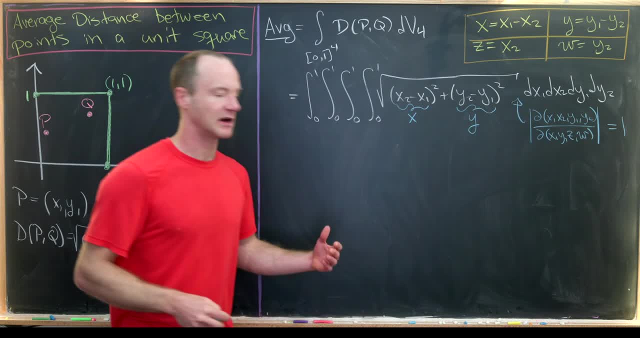 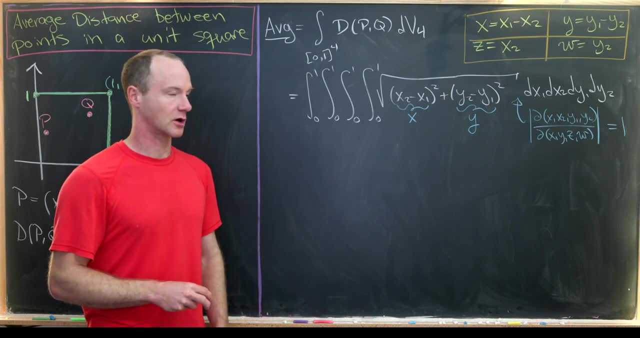 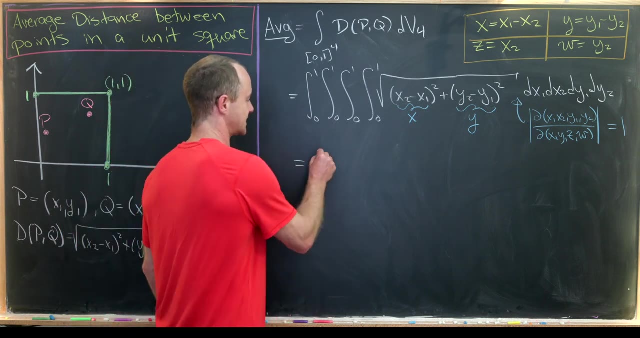 just gives us 1, and it's not exactly the determinant of the Jacobian matrix. it's the absolute value of the determinant of the Jacobian matrix. this comes from the change of variables for Multi variable integrals. okay, so now let's maybe write our next step. so this is going to be the integral over. 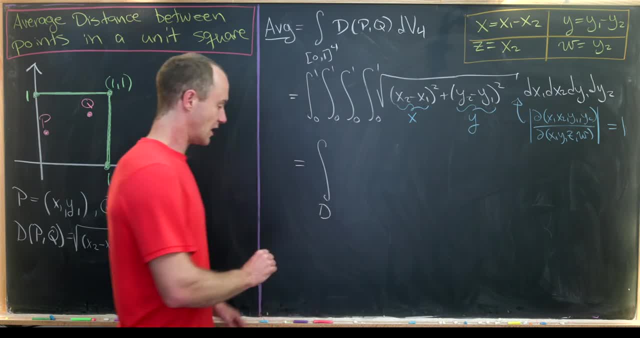 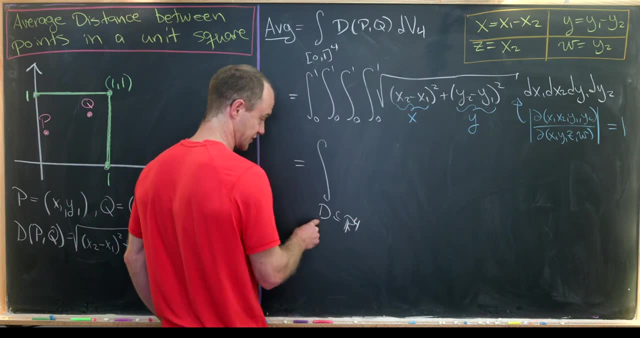 x, y, z squared over x, y squared squared. maybe I'll call this region D, where this region D is our new, like four dimensional region, which is based off of our change of variables. so I'll just say that's a subset of R4 and now we have 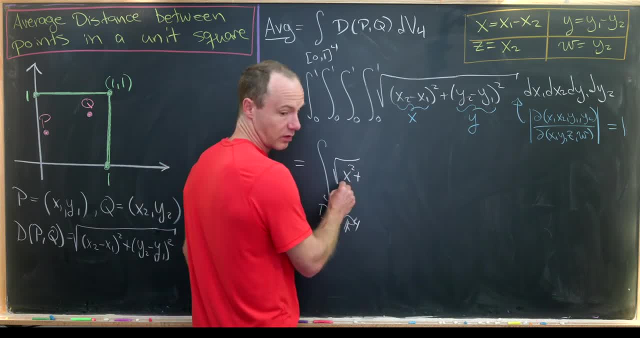 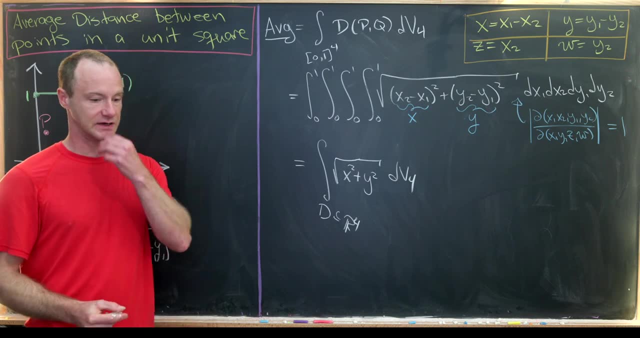 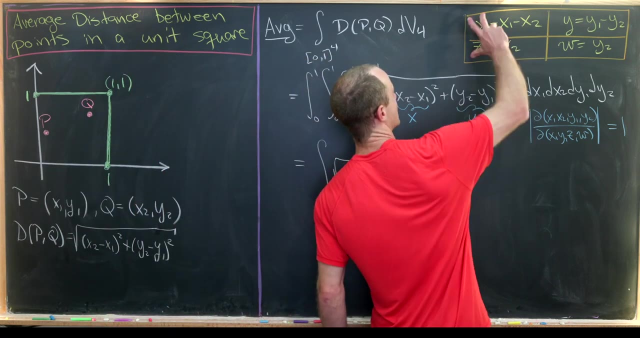 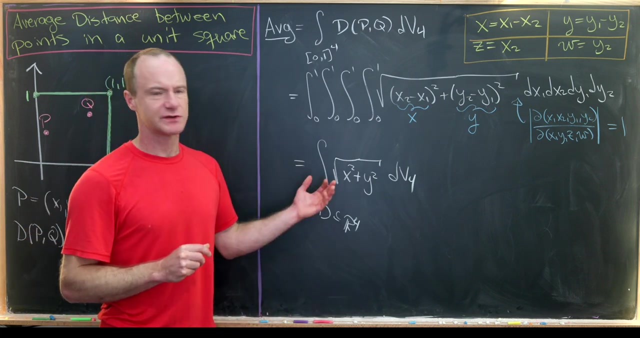 the square root of x squared plus y squared and then another dv4. so we'll have to figure out what that is later. okay, nice. so now note that x1 and x2 are both kind of gobbled up by x and z, whereas y1 and y2 are both gobbled up by y and w. so that means, if we can get a handle on how the x1- x2 unit 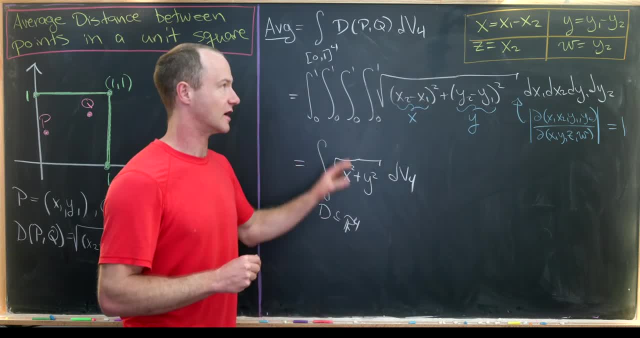 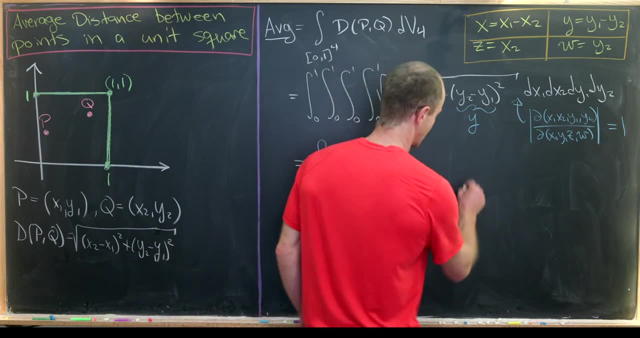 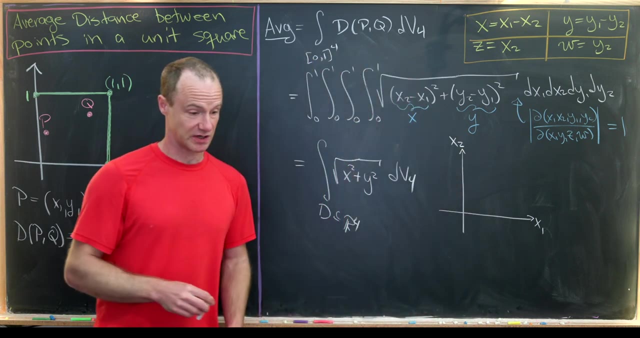 square transforms here, then we know how the integral or the region of the y1- y2 unit square also transforms, okay. so let's make a little bit of a guess here. so let's make a little bit of a guess, a picture of what's going on here. so let's say this is my x1- x2 region. so initially I'm 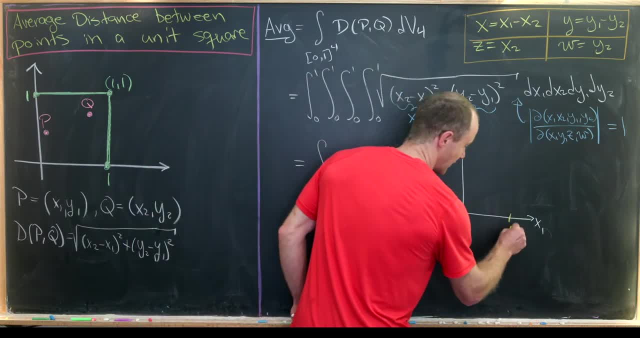 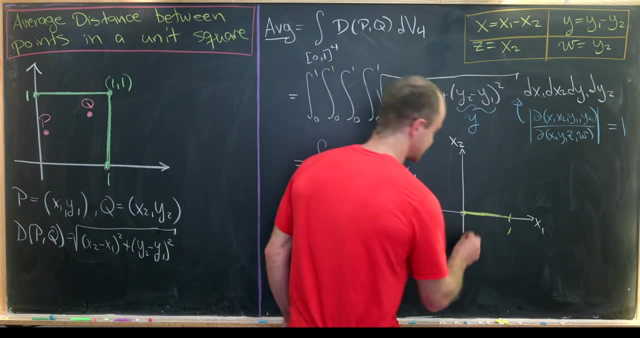 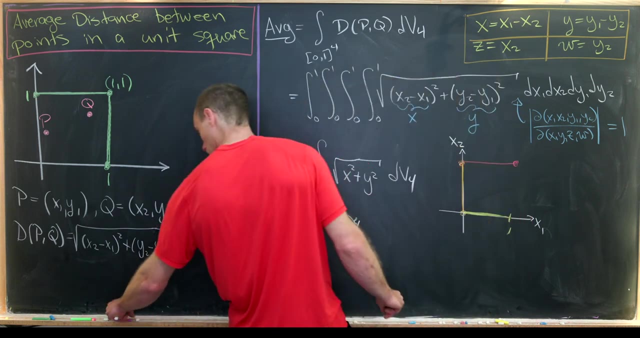 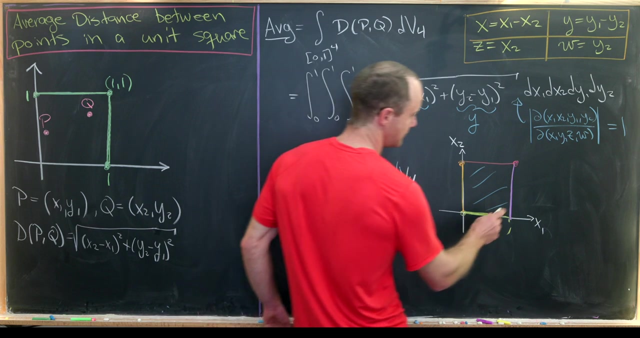 integrating over this region from 0- 1. so, like I said, it's a unit square and I'm going to color code each of these edges, so I'm integrating over all of this region right here. so, and this stuff in the middle. so now our goal, well, our immediate goal is to figure out what this 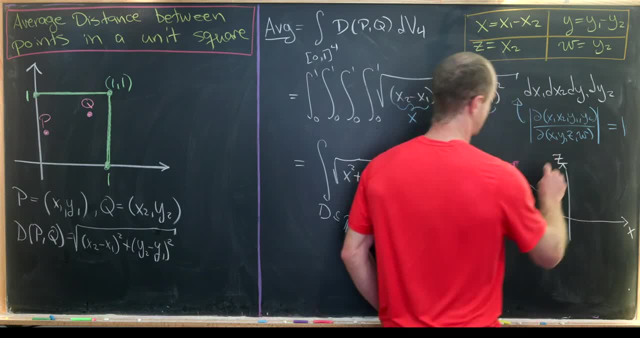 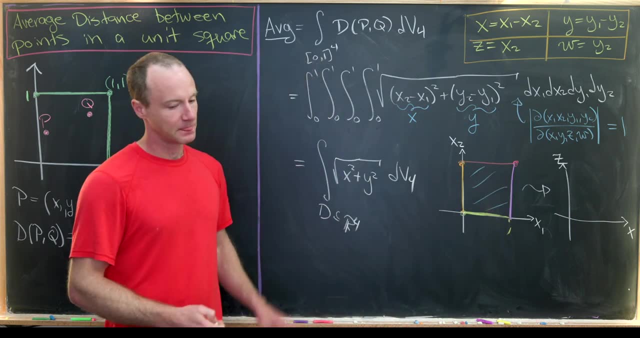 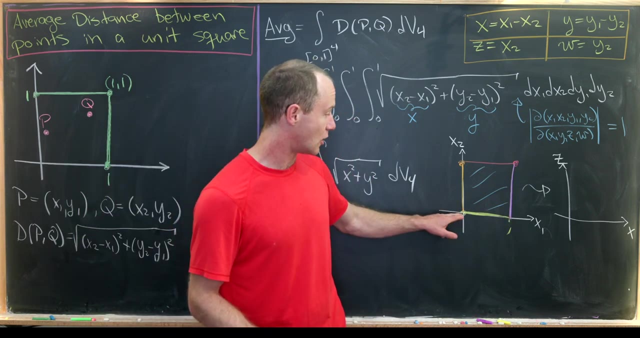 looks like in the x- z plane, and we can do that by seeing what closed curve we get from the boundary here. okay, so let's maybe see how this goes. so if x1 is going from 0 to 1 and x2 is always equal to 0- so that would be this yellow component- then that means that x is going from 0 to 1. 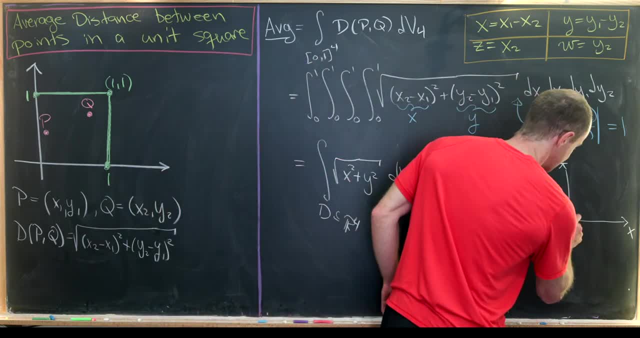 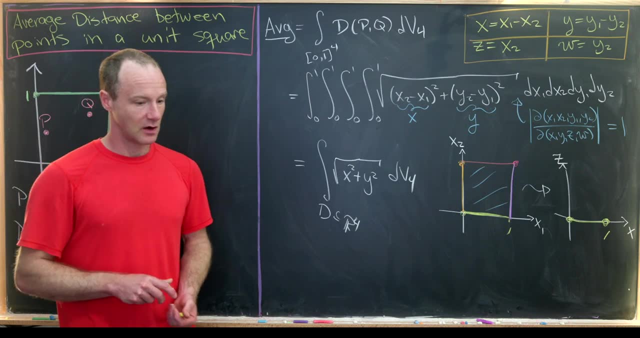 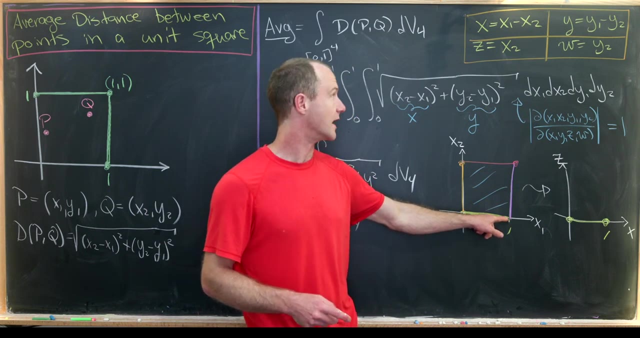 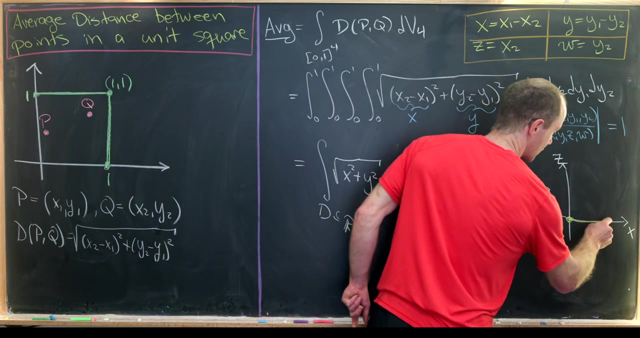 and z is staying at 0, so this yellow turns into this yellow right here. so it's kind of the same line segment. okay, nice, now let's see what's happening over here. so over here, x1 is fixed at the number 1, whereas x2 is going from 0 to 1. so notice, when x2 is equal to 0, we're at this vertex. 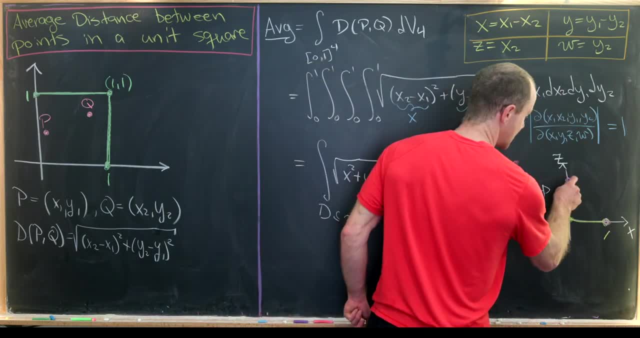 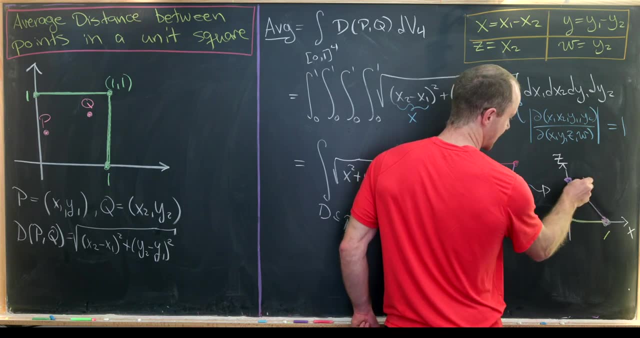 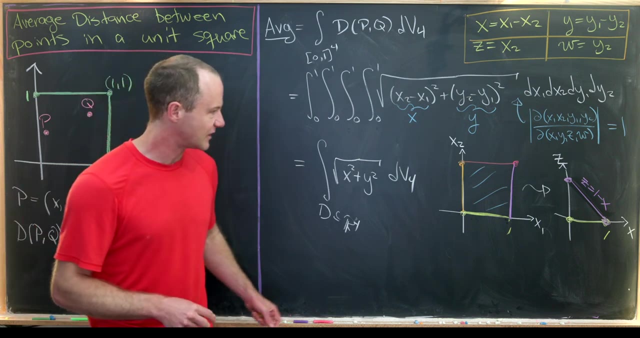 and then when x2 is equal to 1, we're up here, great. so let's maybe make sure that's a line good, and so this ends up being the line: z equals 1 minus x, which isn't too hard to check. okay, so that's looking good. now let's figure out what's. 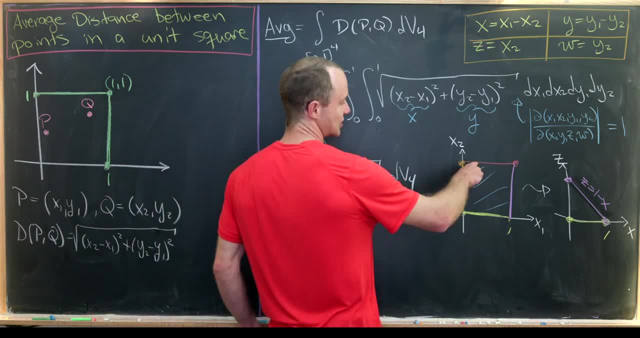 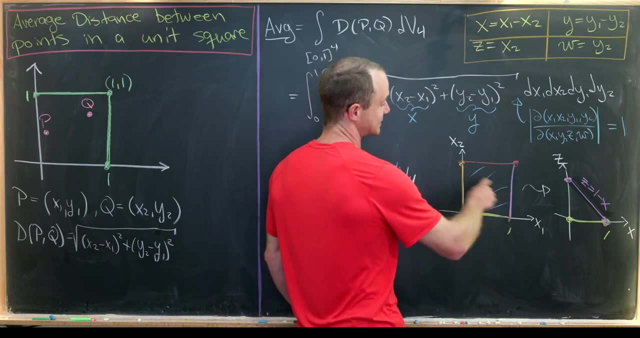 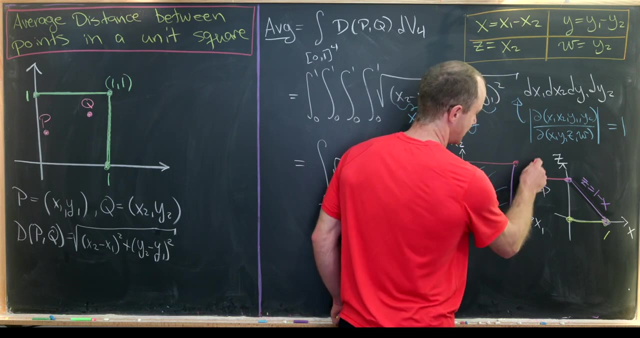 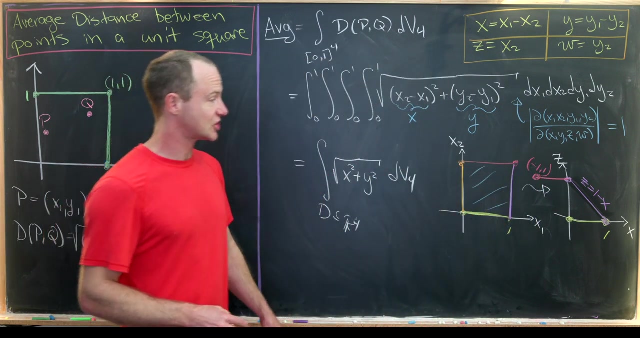 going on on with the other parts. so this region up here, or this red line segment, I should say, that's when x2 is fixed at 1, whereas x1 ranges between 0 and 1. so that's going to give us, like this, back here to this point, let's see negative 1, 1 and then finally, to finish it all, 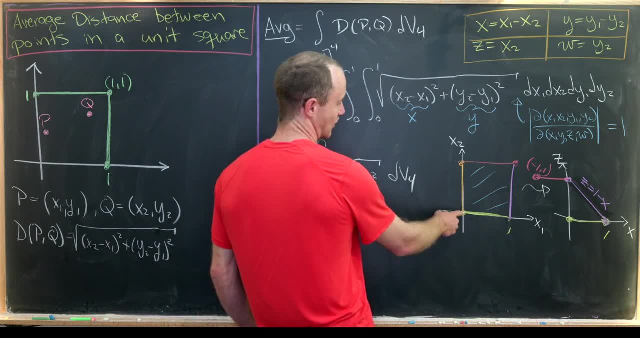 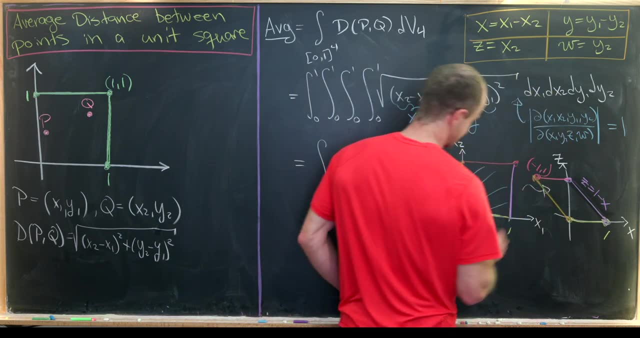 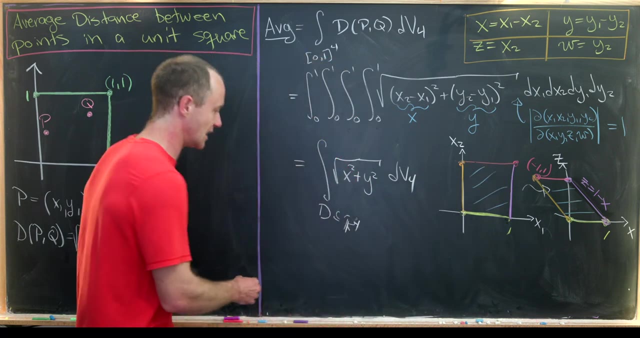 off this region right, or this line segment right here, where x1 is equal to 0 and x2 is trending between 0 and 1. we'll finish this thing off. so we've got this parallelogram over here. so this is the region that we're integrating over. so now, keeping this picture in mind, we can rewrite this. 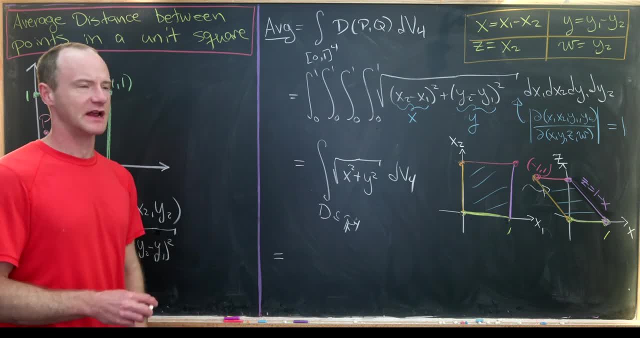 integral, this like 4 integral, and then we're going to have this line segment right here where x1 is equal to the integral, to the integral, as an iterated integral, where we've got two integrals on the outside and two integrals on the inside, so it's going to be the integral from 0 to 1. 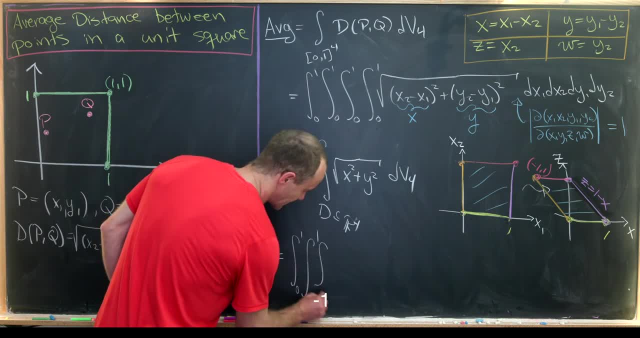 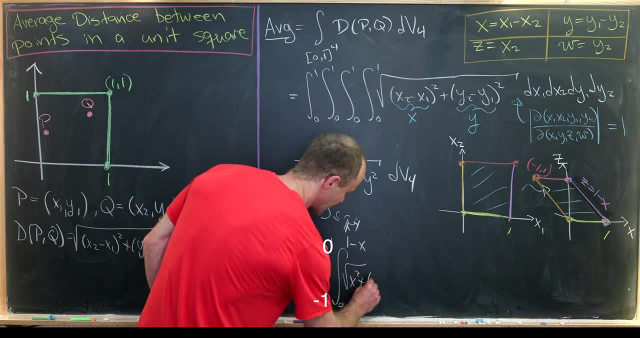 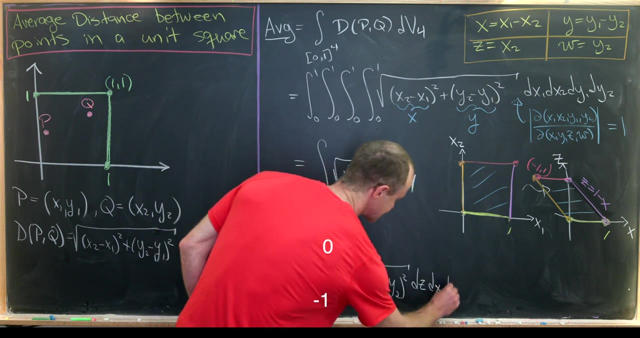 the integral from 0 to 1, and then the integral from 0 to 1, and the integral from 0 to 1 minus x, of the square root of x squared, plus y1 minus y2 squared, and then here we have dz, dx, dy1, dy2. 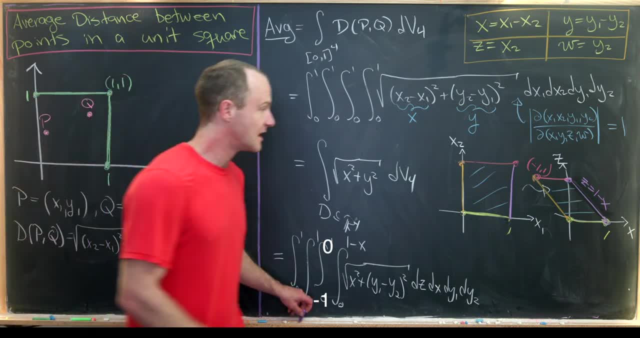 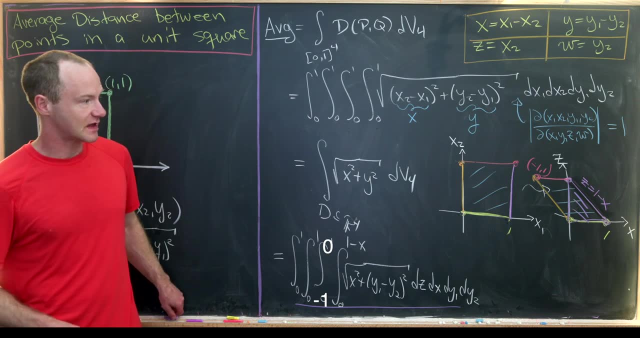 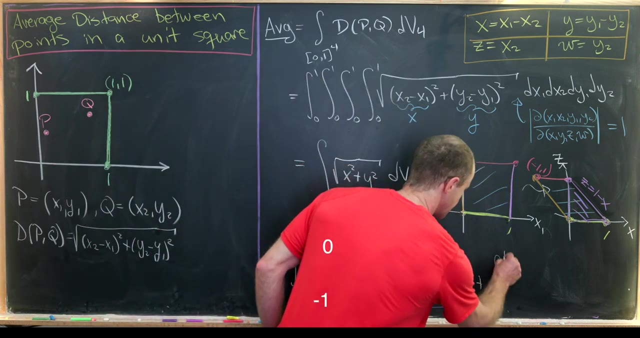 so that doesn't capture everything over there that captures what's going on right here. so this triangle right here, okay, so that means we need to add on this other triangle, so that's going to end up being plus the integral from zero to one, zero to one, zero to one, and then now we're going from. 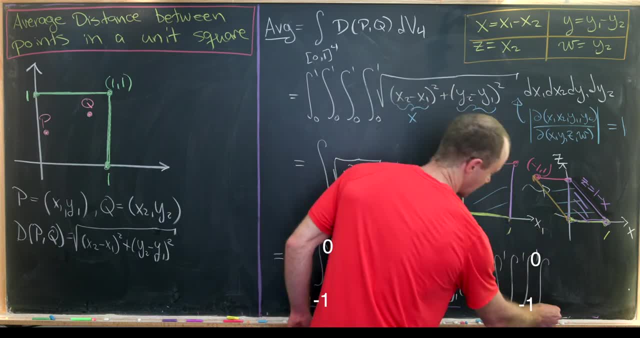 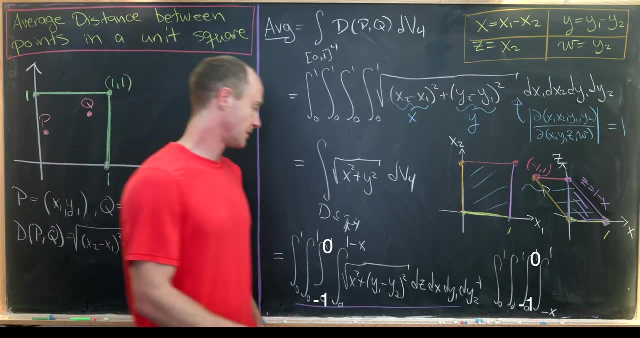 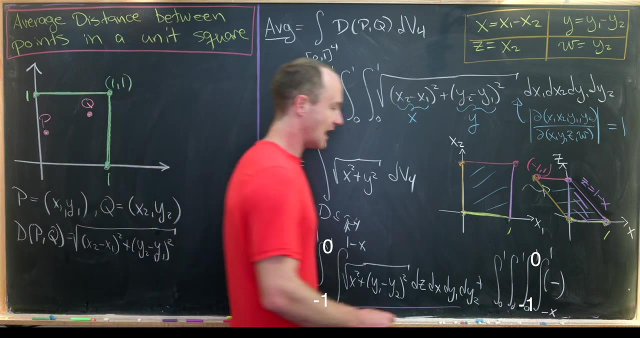 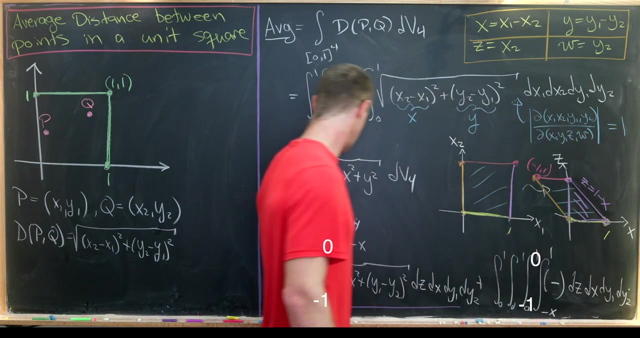 let's see that our lower component or our lower curve is negative x up to the number one. so that would be this upper red curve of the same function here. so i'm running out of room so i'll just put kind of parentheses for that same function and then we'll have again dz, dx, dy1, dy2. okay, so that's. 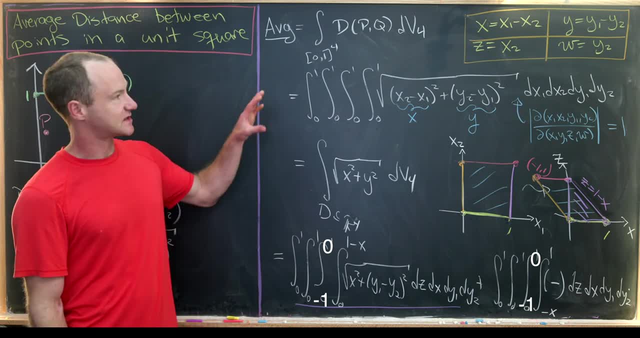 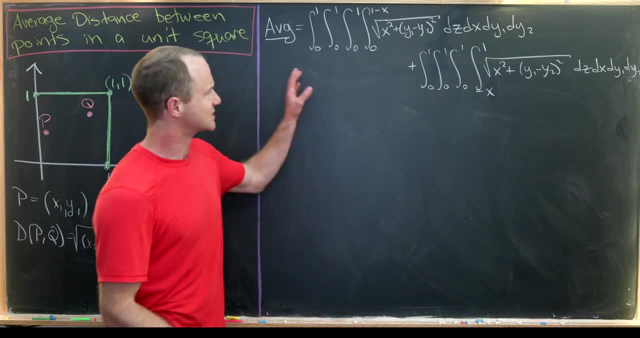 where we are after all of this calculation. so let's summarize that at the top and then we'll keep going. so this is where we left ourselves. so our average, which is kind of our goal, was equal to the sum of these two quadruple integrals. but notice the inner. 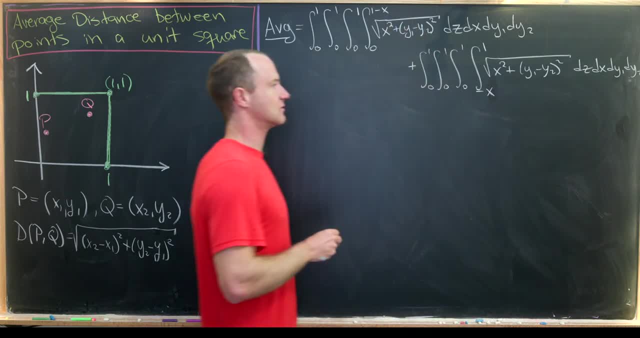 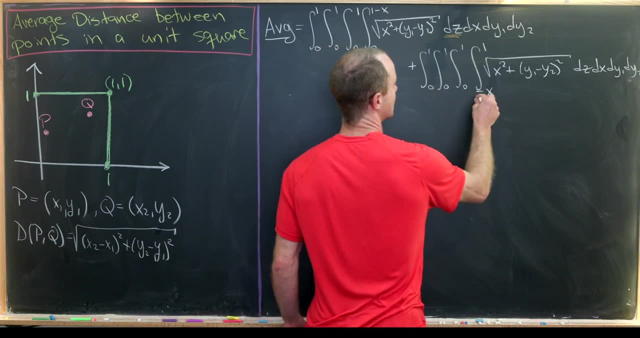 function does not depend on z, which is our innermost integral. that means the innermost integral is fairly simple. so let's take care of each of these inner integrals first and see what that leaves us with. so this first one is going to collapse to the integral from. 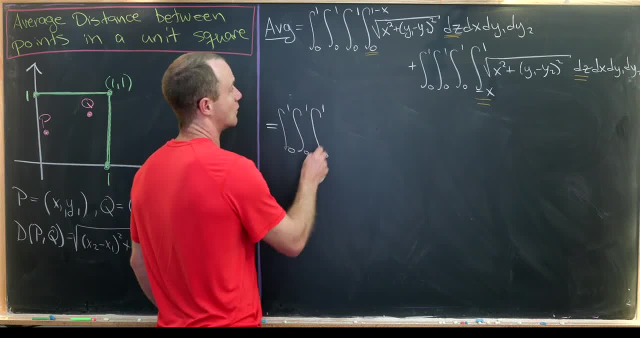 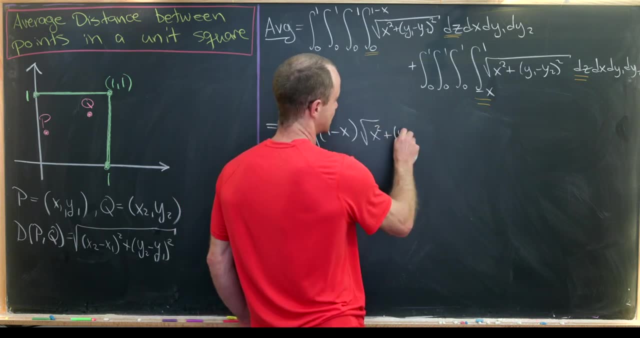 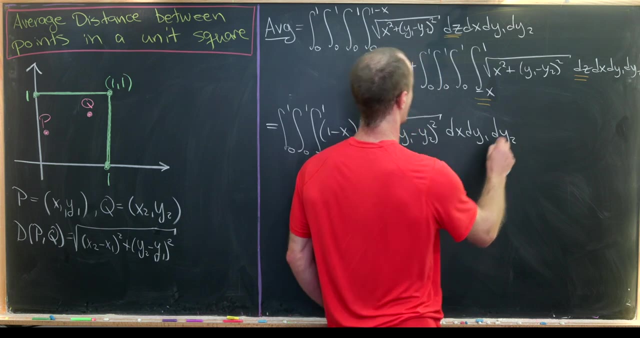 zero to one, zero to one, y andอ 0 to 1, and then another 0 to 1 of 1 minus x times the square root of x squared plus y1 minus y2 squared, And then we have dx, dy1, dy2.. Again, that's from this z integral. 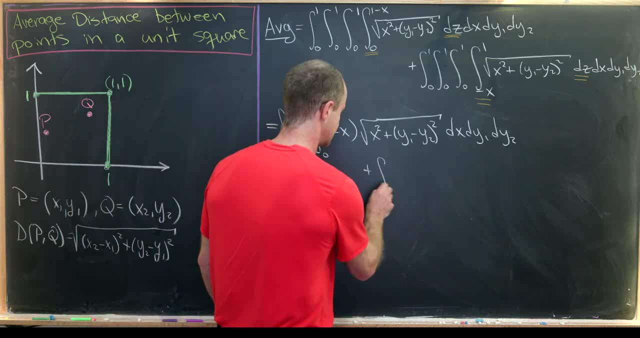 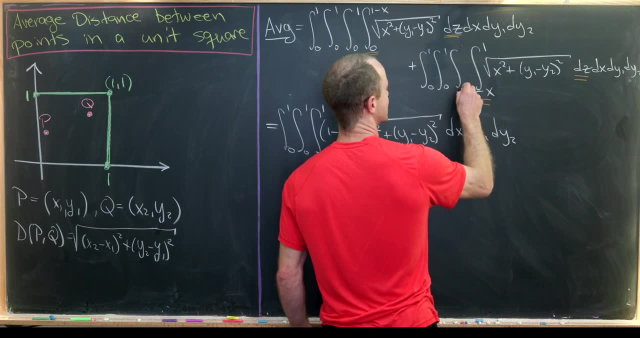 And then next we'll have plus the integral from 0 to 1, 0 to 1, 0 to 1.. Oh, and I realized I have a typo right here. That should have been minus 1 to 0, because those are the x bounds of. 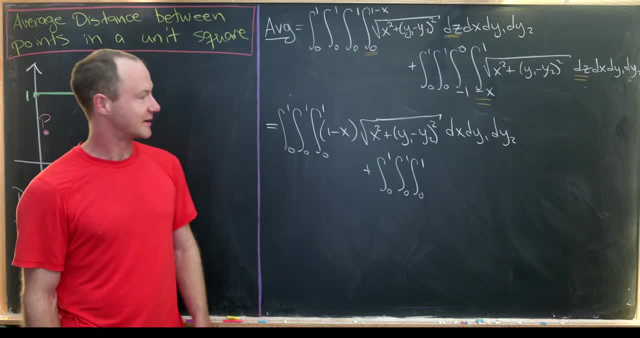 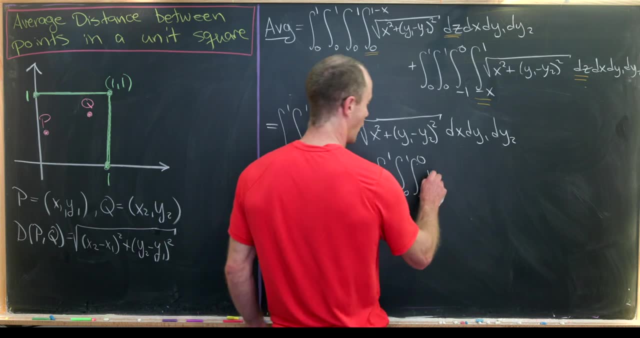 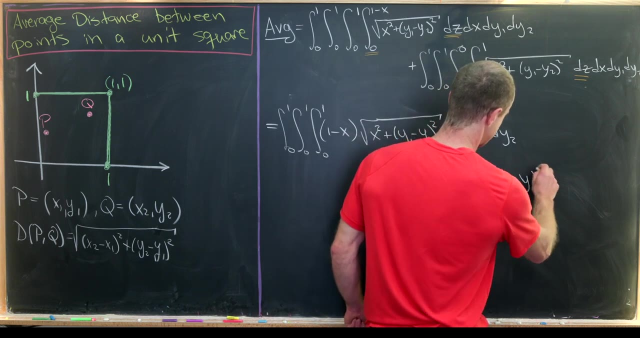 integration. The editor will fix that on the last board, so don't worry about it. Okay then. so, like I said, this is going to be minus 1 to 0, and then we'll have 1 plus x, and then the same function, x squared plus y1, minus y2 squared, and then we have dx, dy1, dy2.. 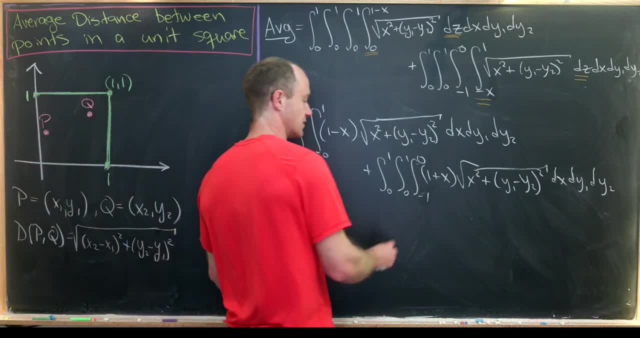 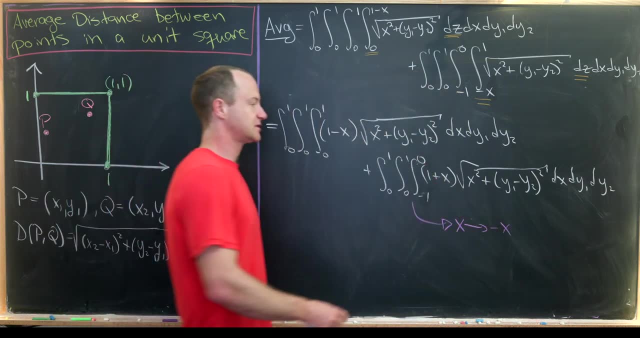 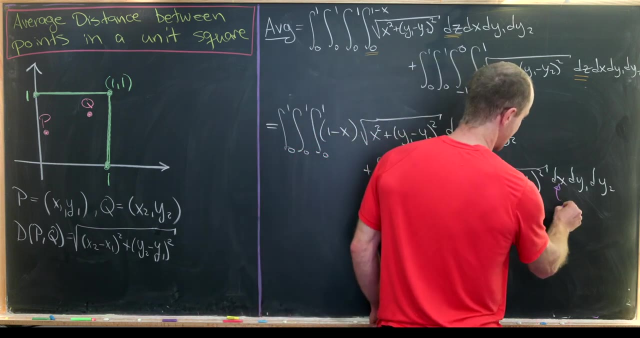 Now we'll do a kind of more trivial change of variables here, and that change of variables will be to replace x with minus x, So that's going to turn this into a minus x, and then this is going to go from 1 to 0, and then this dx is going to turn into minus dx, which will change. 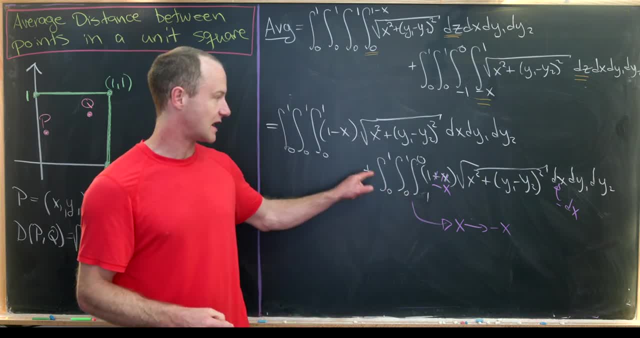 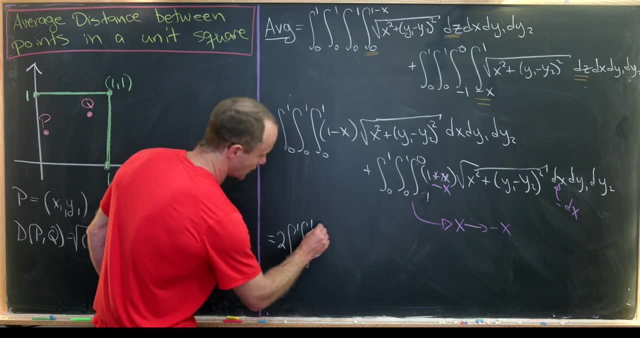 the bounds of integration here, allowing us to combine this integral with the one above, giving us 2 times dx dy2.. So that's going to be 1 times this triple integral: 0, 1, 0, 1, 0, 1, 1 minus x, and then we have the 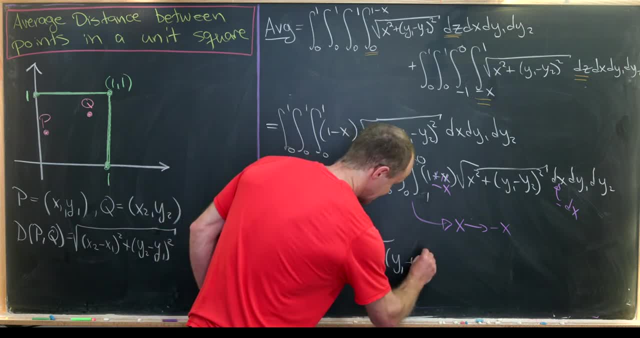 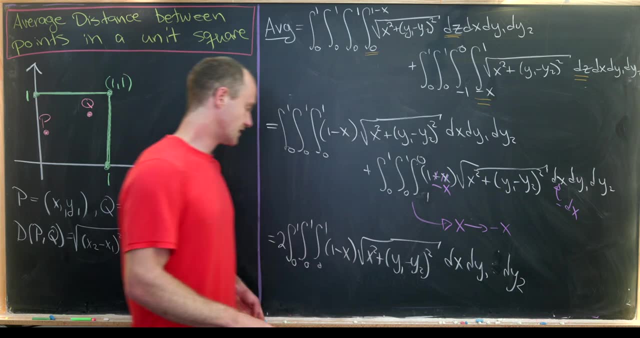 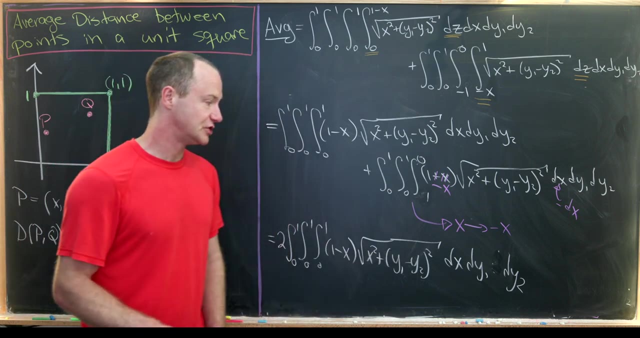 square root of x, squared plus y1 minus y2, squared dx, dy1, dy2, like that. And now, indeed, we can do the same kind of thing with y1 and y2 variables that we just did with the x1 and x2 variables. 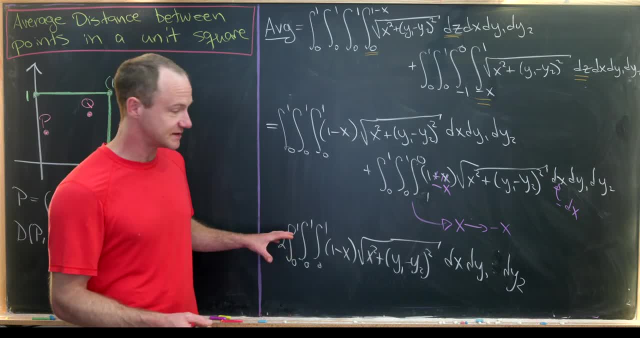 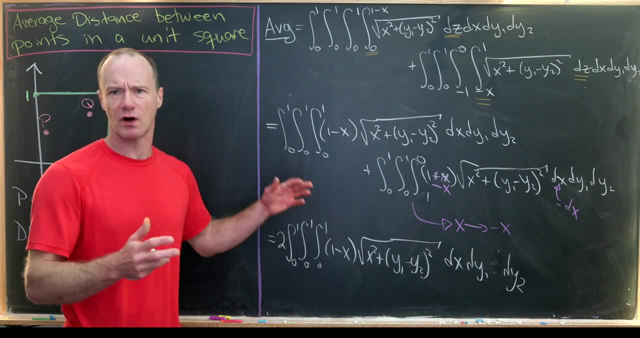 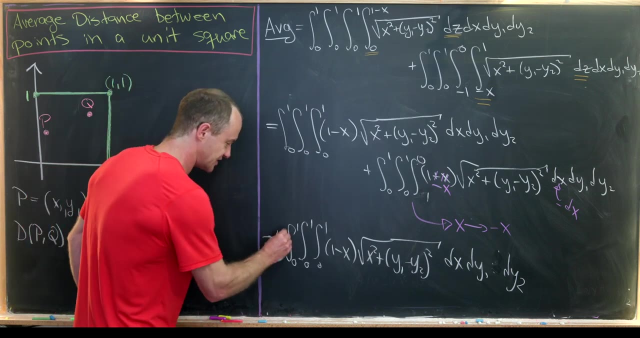 and we're going to pick up another 2, as well as a 1 minus y out front as we collapse. this y1 minus y2 just to y. So again, this is essentially exactly the same thing we did already, so that's going to change. 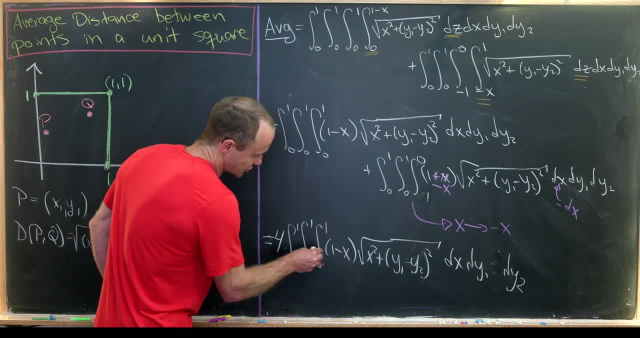 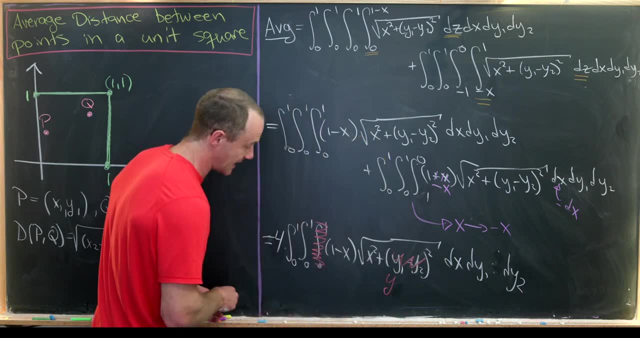 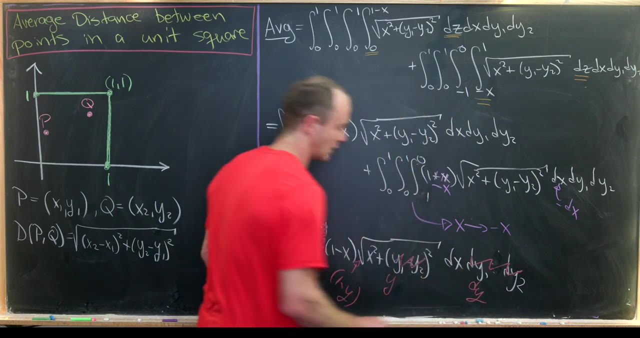 this into a 4. It's going to collapse this triple integral into a double integral. It'll collapse this y1 minus y2 just to y, and it'll also insert a 1 minus y here and it'll collapse this dy1, dy2 just to dy. So we're left with a kind of more friendly double. 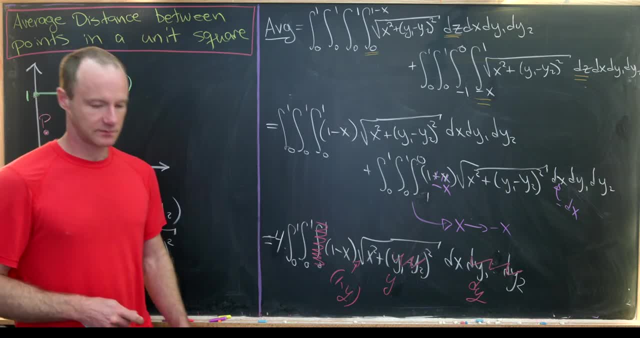 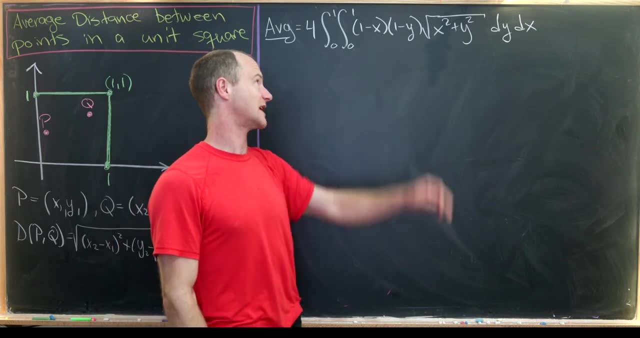 integral. So now let's get to work on that double integral. So this is where we left ourselves. on the last board, Our average value we're looking for was 4 times this double integral of 1 minus x, times 1 minus y, times the square root of x squared plus y squared. Now this x squared plus. 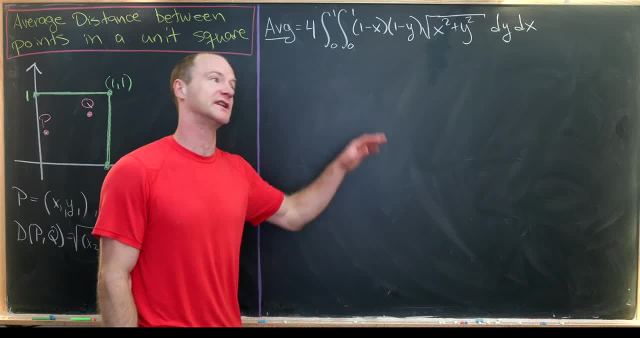 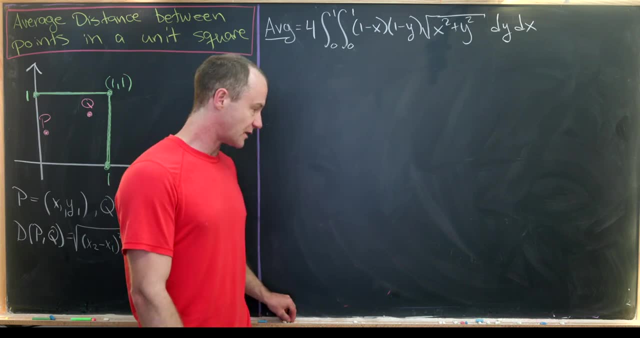 y squared gives us motivation to use something like polar coordinates. However, the fact that integrating over a square kind of pushes us against polar coordinates, So I think you can do this kind of appropriately with or without polar coordinates. We're going to do it maybe. 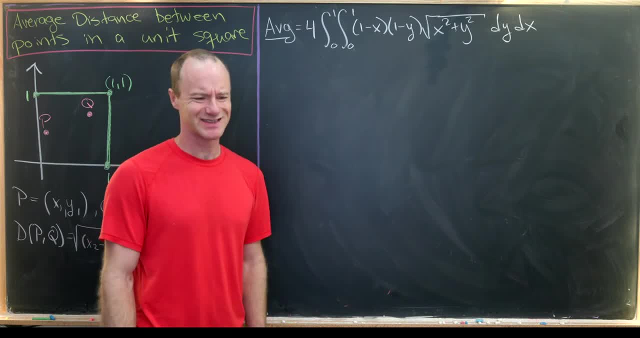 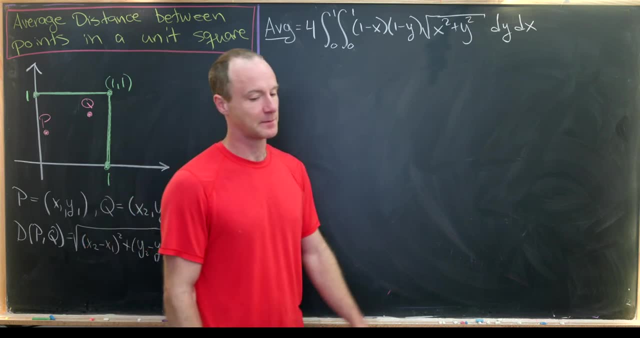 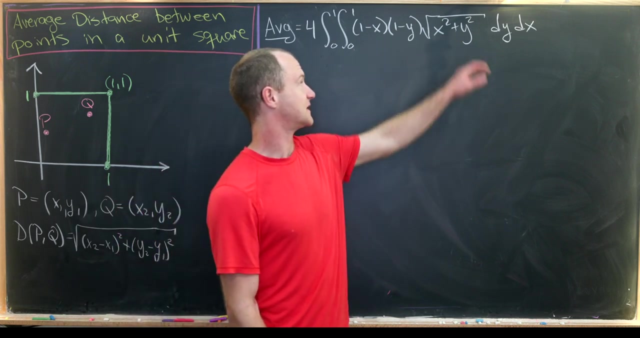 without polar coordinates but with a trig change of variables, which is kind of the same thing. I think that probably all of these paths are about the same type of difficulty. Okay, so we're going to focus on the inner integral first, which is with respect to y, and we've got this x squared. 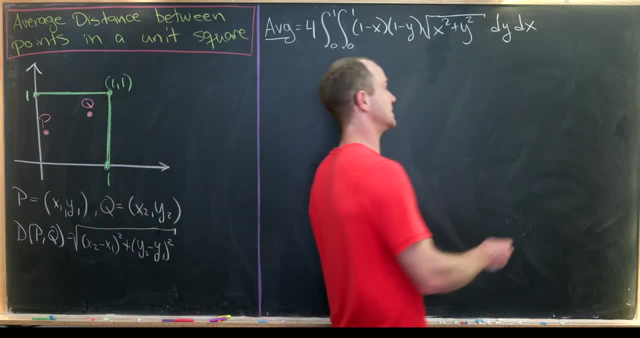 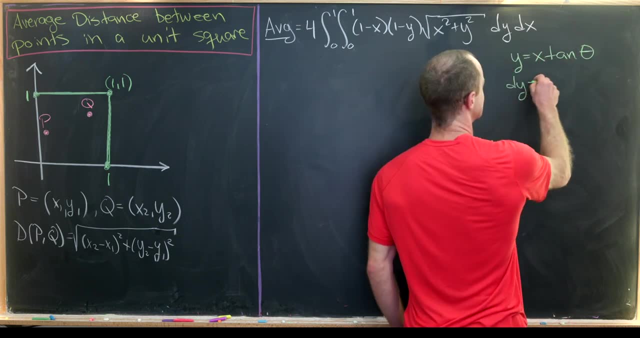 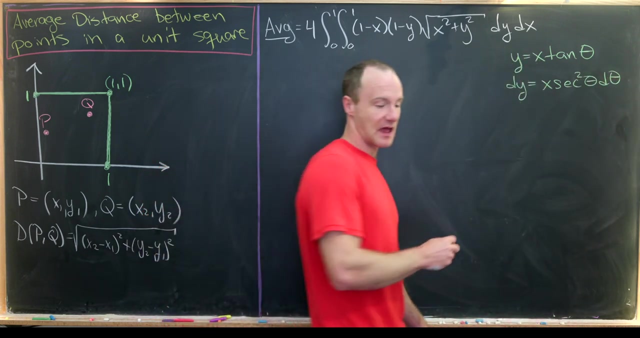 plus y squared, which minus y squared. So we're going to do this kind of appropriately with or motivates a tangent substitution. So let's set y equal to x times tangent of theta. That means that dy is x times secant squared theta d theta, And then that means that x squared plus y squared. 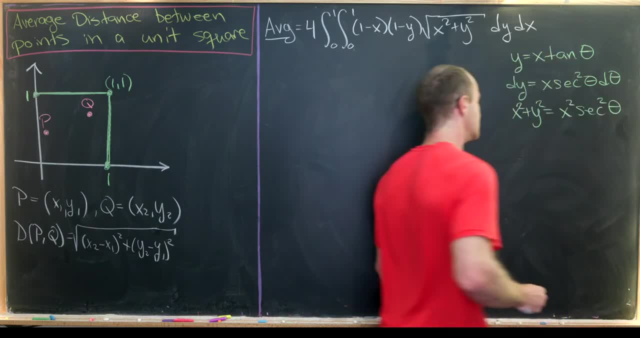 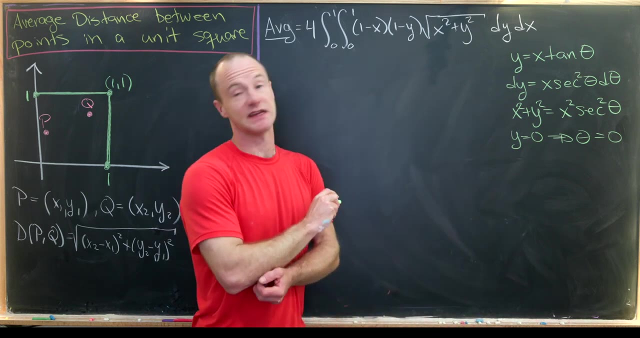 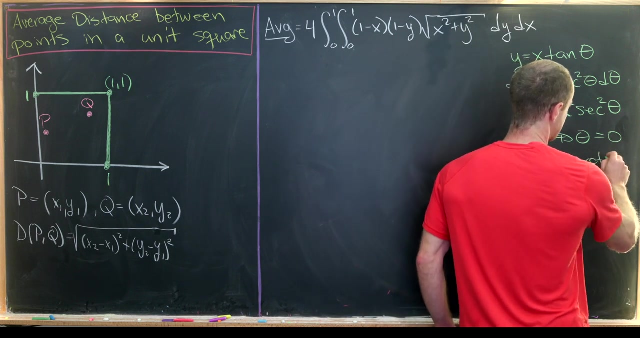 is x squared times secant squared theta. So that's by like trig identities: If y is equal to zero, that implies that theta is equal to zero. So that's because tangent of zero is zero. And then if y is equal to one, that means that theta is equal to the arctan of one over x. 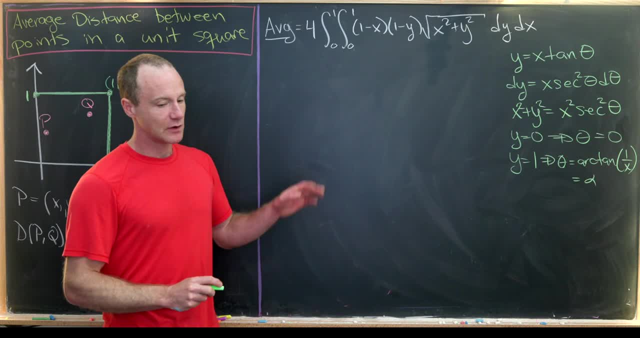 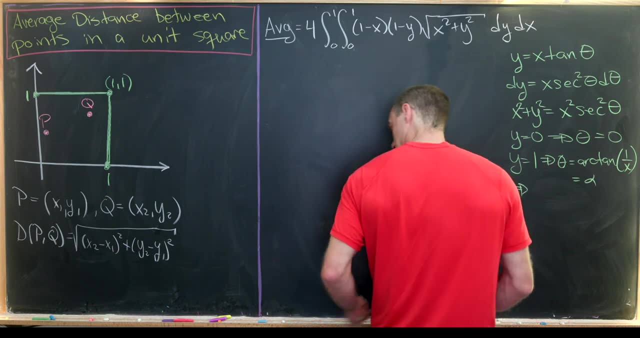 We'll just call that number alpha. Then we need one more thing. So if alpha is equal to the arctan of one over x, that means that the tangent of y is equal to one over x. So we're going to do this. 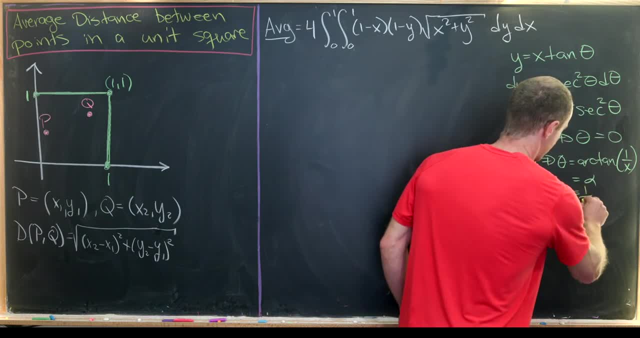 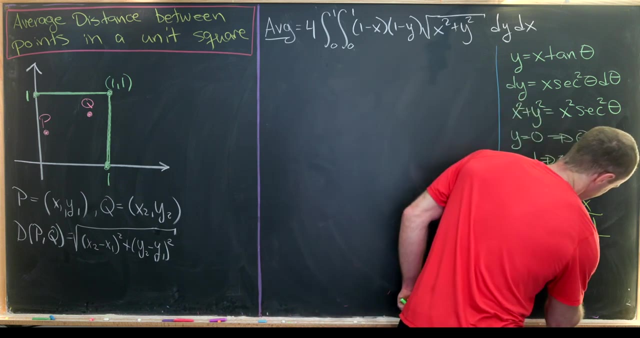 the tangent of alpha is equal to one over x, which means the secant of alpha using trig identities is equal to the square root of one plus x squared over x. So we're going to need that as well. Okay, so there's all our like kind of long work in order to set up this trig substitution. 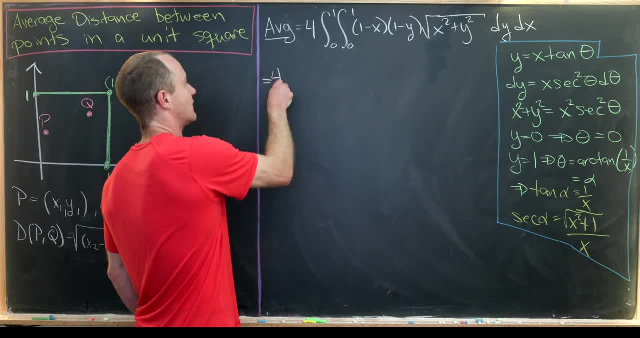 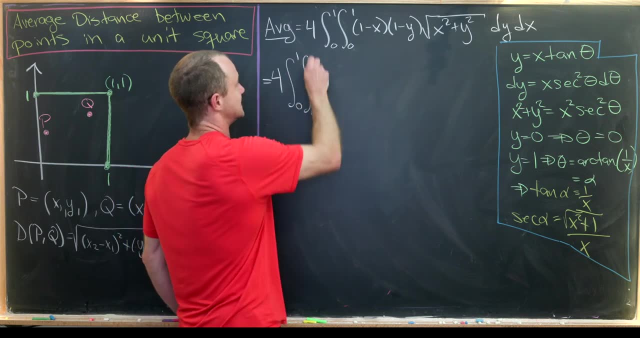 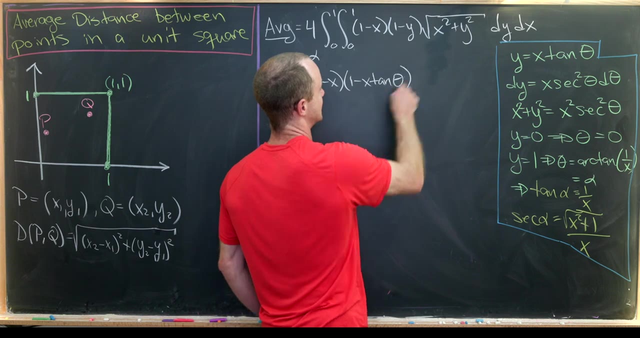 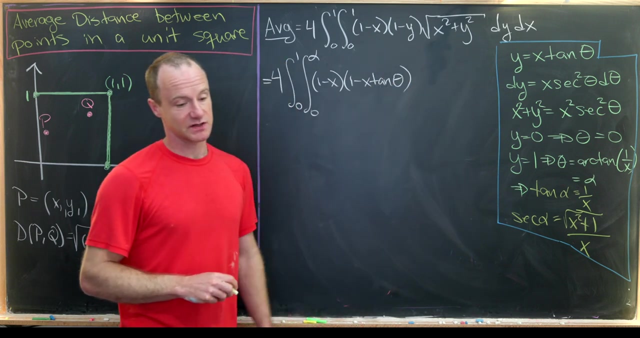 Okay, so let's see what that leaves us with. So we're going to have four. then the integral from zero to one, the integral from zero to alpha of one minus x, one minus x times tangent theta, And then here we've got x times secant theta after taking the. 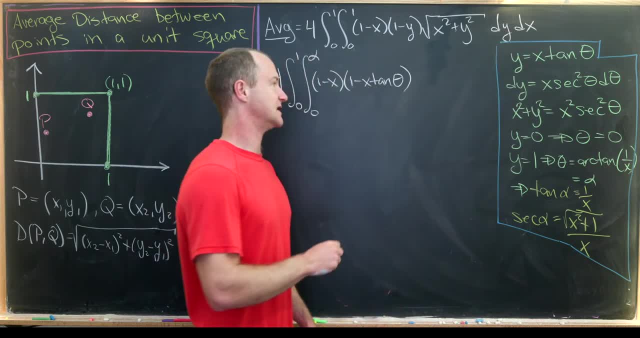 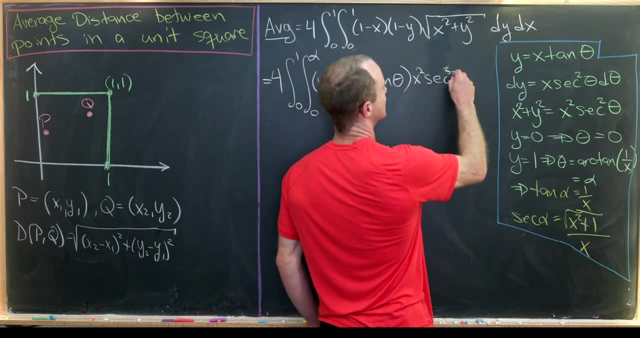 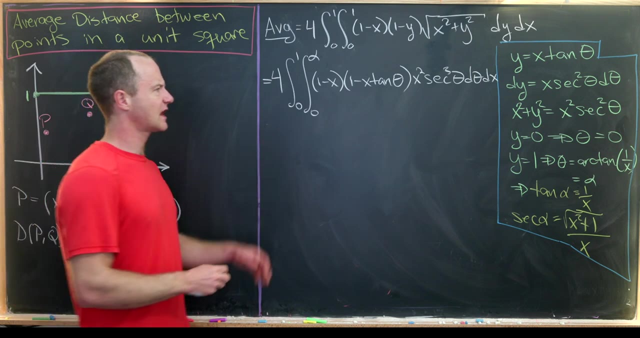 square root, and then an x times secant squared theta from the dy, leaving us with x squared times secant cubed theta. And then we have d theta, dx. So we have something that looks like that. Okay, so now let's rewrite. 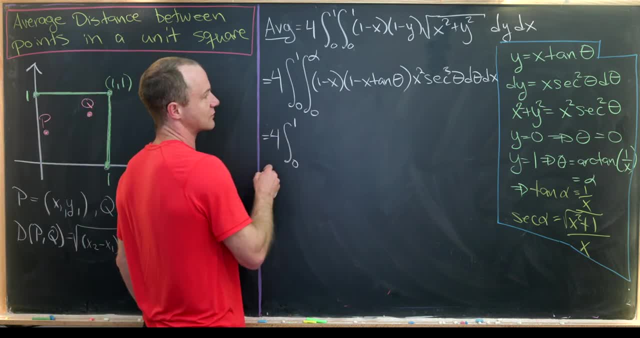 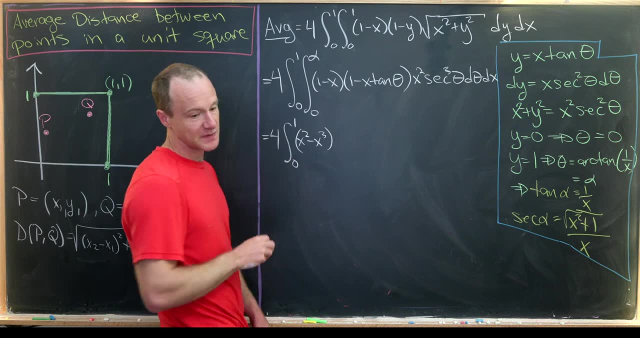 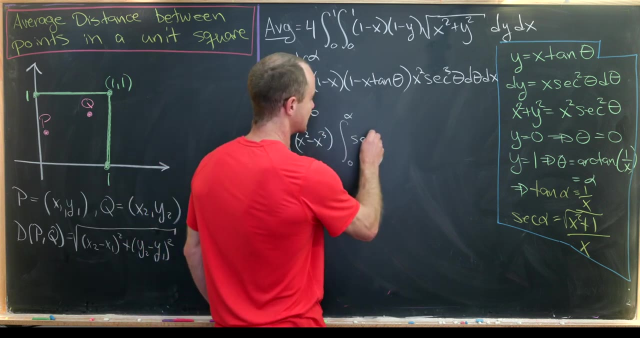 this a little bit. That's going to give us four: the integral from zero to one of x squared minus x cubed. That's this part that depends on x. And then, inside of this x integral, we have the integral from zero to alpha of secant cubed theta, and then minus x times secant cubed theta. 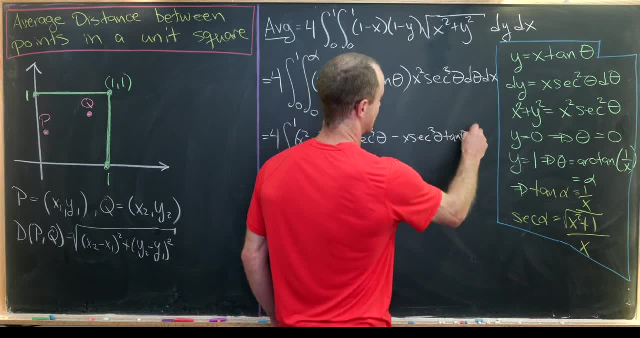 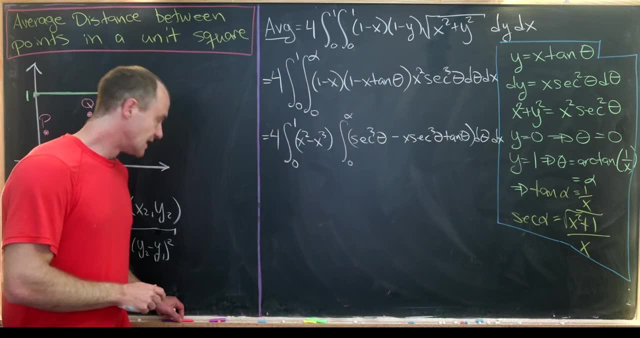 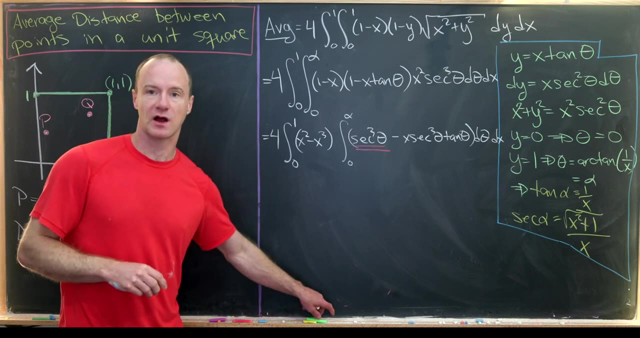 times secant cubed theta, tangent theta, And then this is all d theta And then outside of all of that is a dx term. Now this secant cubed theta is kind of a classic integral. So I've calculated it on the channel many times before. I won't calculate it again, We'll just jump to what it is And then 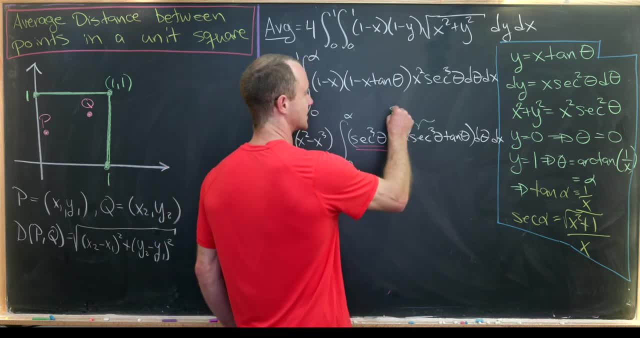 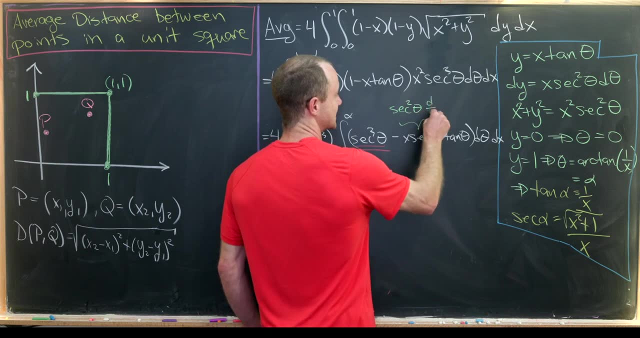 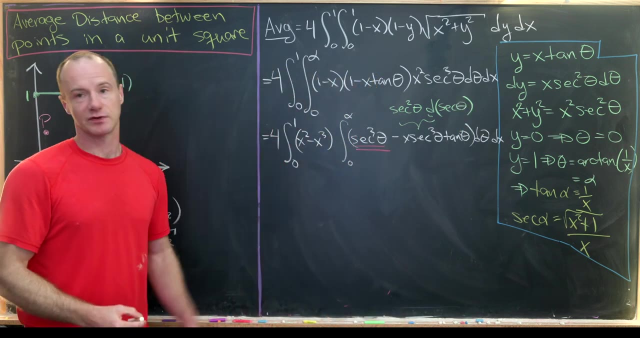 the secant cubed theta, tangent theta is actually quite a bit easier because this is secant squared theta times secant theta, tangent theta. But secant theta, tangent theta is the same thing as the differential of secant theta. So we have a nice change of variables that allows us to calculate. 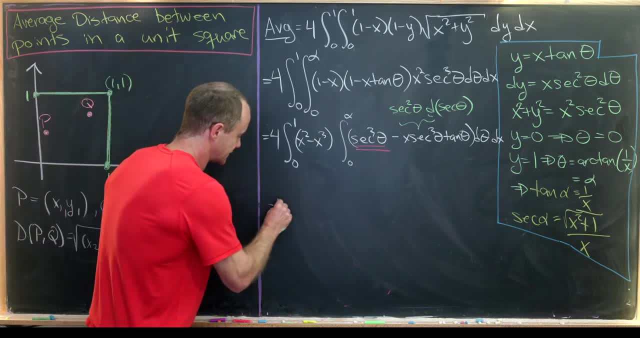 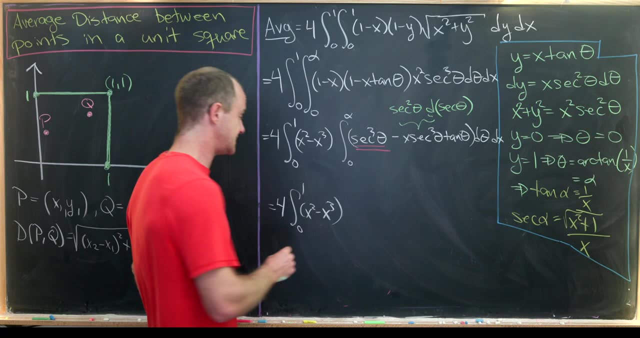 that Okay. so anyway, that's going to leave us with four. And then the integral from zero to one of x squared minus x cubed. This secant theta turns into one half. Sorry, secant cubed theta, Secant theta, tangent theta. And then the integral from zero to one of x squared minus x cubed, And then 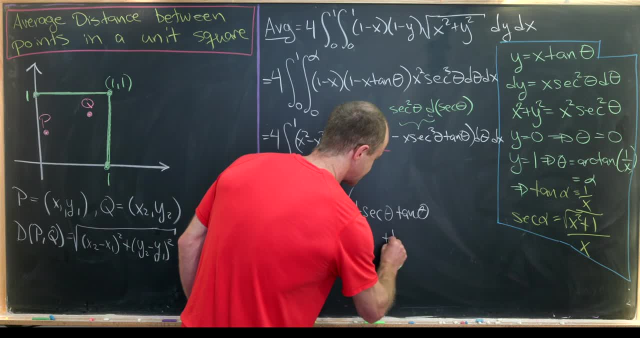 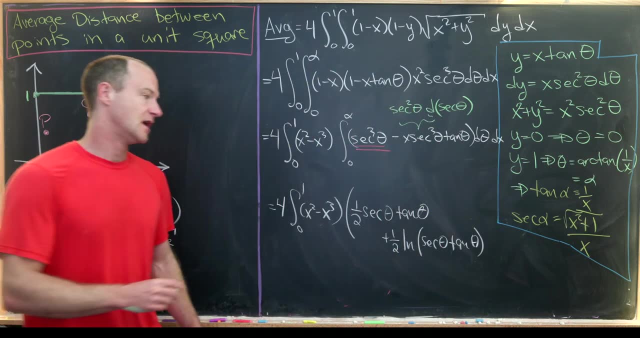 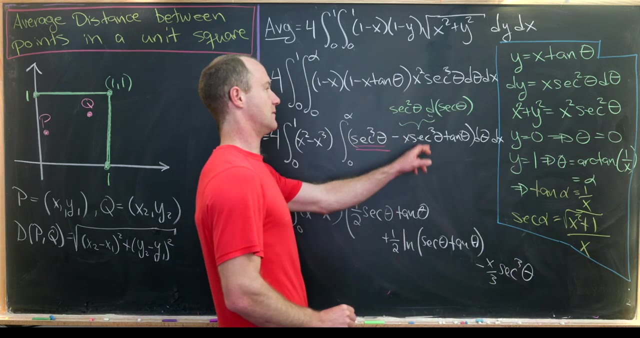 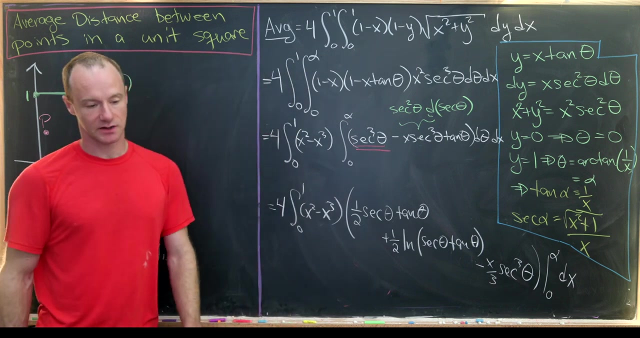 plus one half the natural log of secant theta, tangent theta, Like that, And then we finally have a minus x over three times the secant cubed theta from this one right here. Then we need to evaluate that all from zero to alpha And then we've got a dx here. Okay, so if we plug alpha into all of 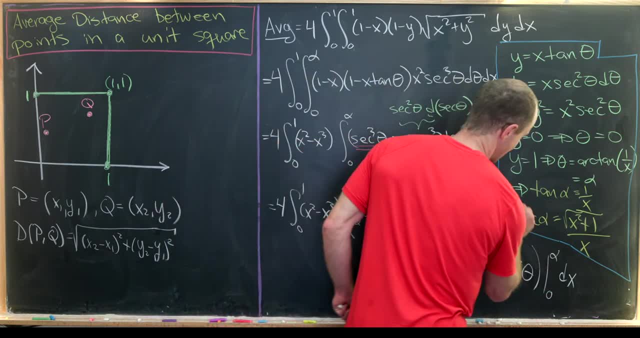 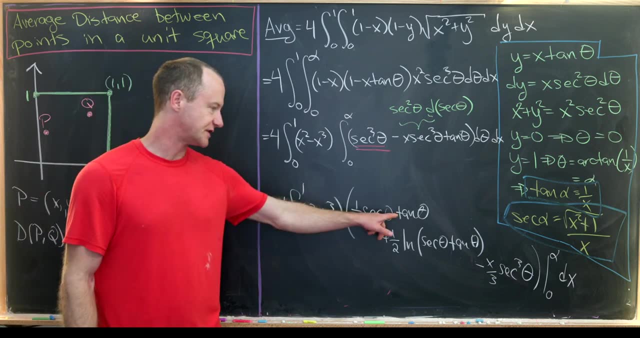 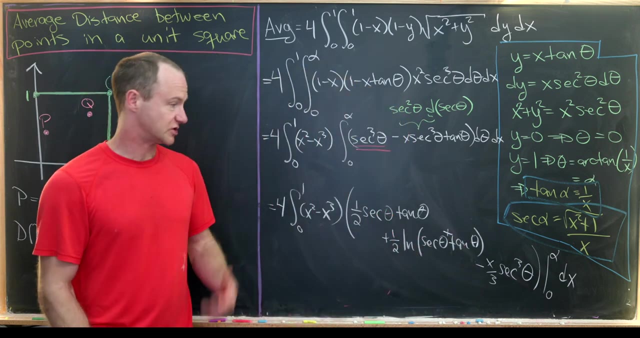 these trig functions We get these values as described over here. So there's our secant, There's our tangent, And then if we plug zero in, Well, tangent of zero is zero, So this cancels. That should be natural log of secant plus tangent. So that gives us natural log of one which is 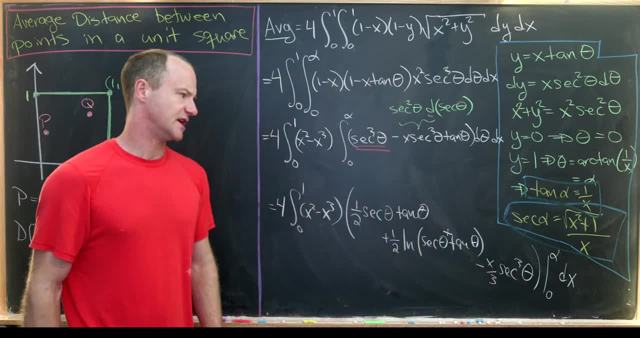 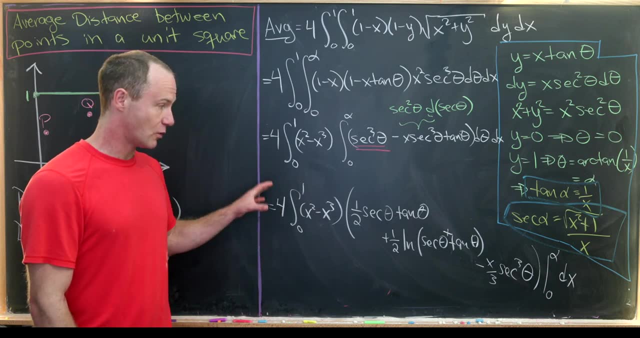 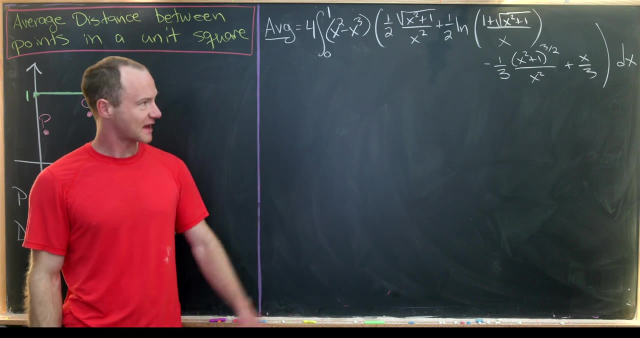 zero, And then secant of zero is one. So that's how that simplifies. Okay, so let's jump to that on the last, on the next board, with just an x integral, And all of this is going to be substitutions made as described by these. So after all of that substitution, we get the following: 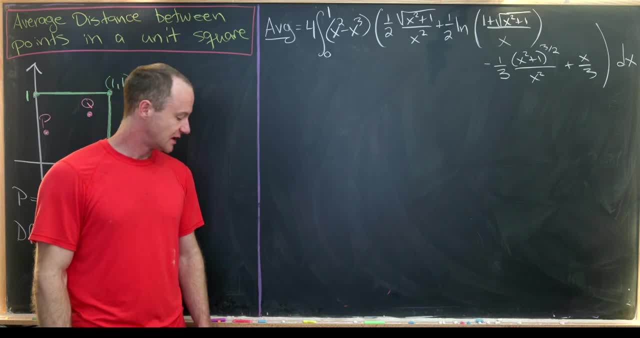 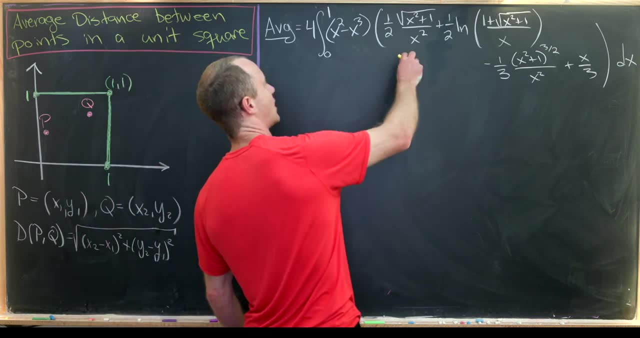 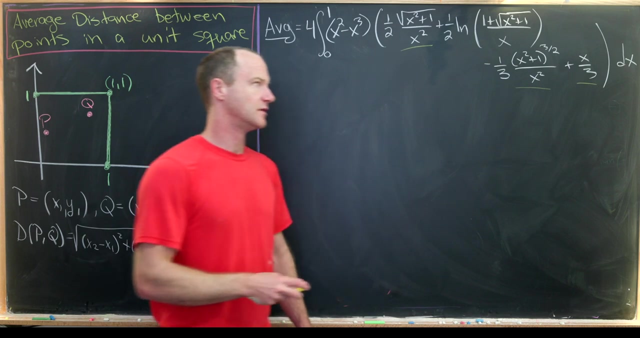 single integral which only depends on x. Now portions of this single integral are fairly straightforward to calculate, Like, for example, if we take this polynomial into this radical expression or this radical expression or into this polynomial. Those vary in difficulty But I think you would calculate all of those with trigonometric substitution. 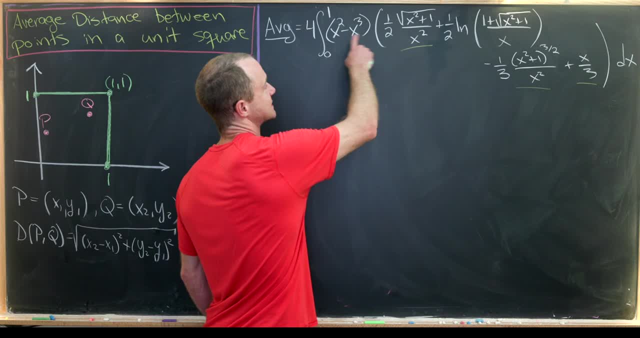 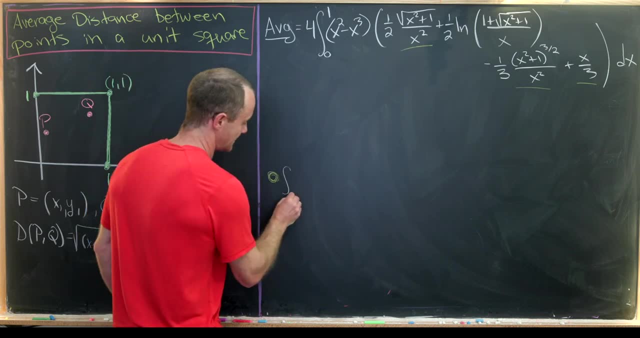 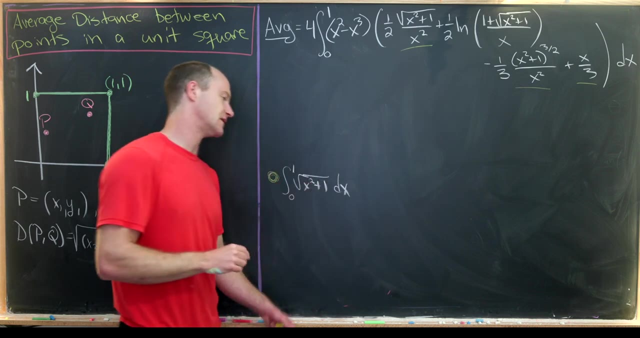 So like, for instance: if we multiply x squared into this x squared in the denominator, We have an integral that looks like this: to calculate The integral from zero to one of the square root of x squared plus one dx, We can make another tangent substitution here. So x is 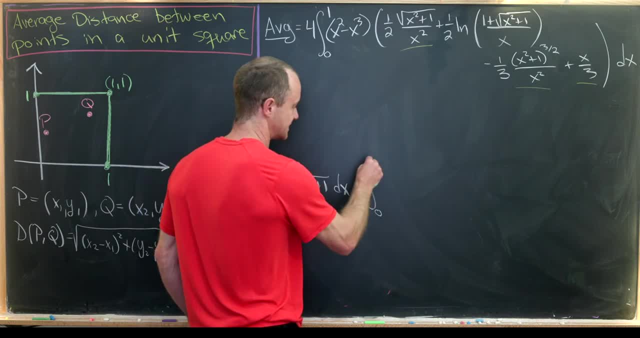 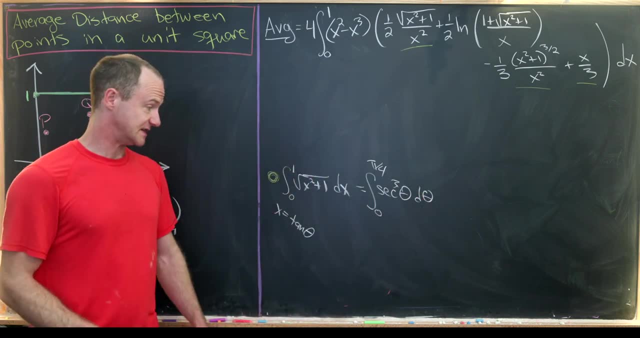 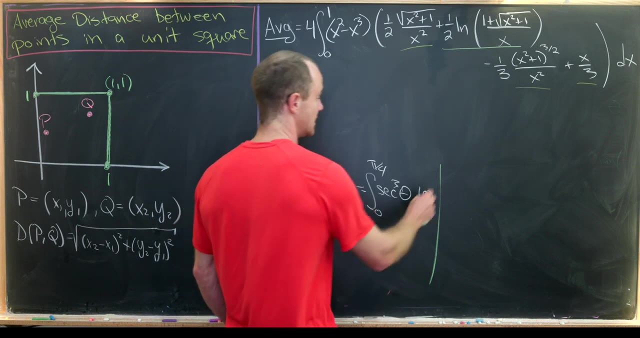 tangent theta And that actually turns this into the integral from zero to pi over four of secant cubed theta dx, And I won't work out the details on that. But if we look at this guy right here, this one is actually quite complicated And notice there are two terms connected to this. There's the x- cubed and the x.